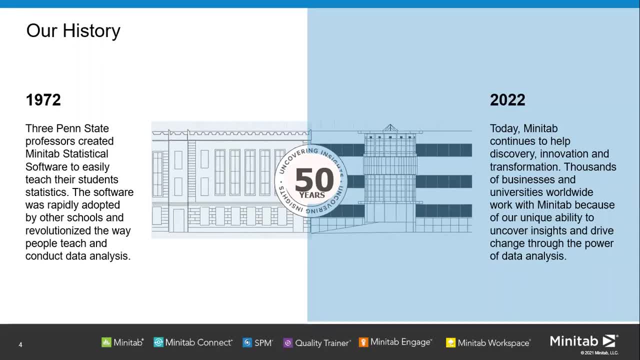 1972.. So today Minitab in market for 50 years. Minitab statistical software is a software package for statistical analysis, So variety of statistical tools are available in Minitab, This software. it will be powerful statistical software since everyone can use, whether you. 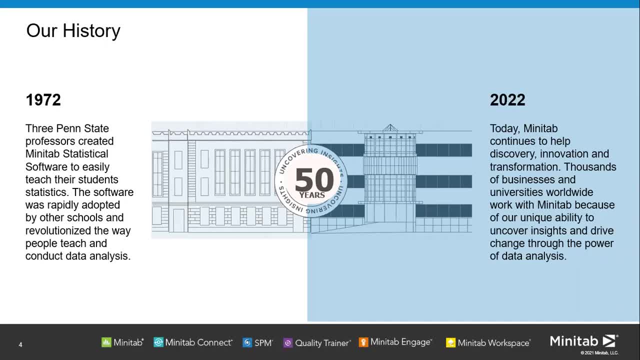 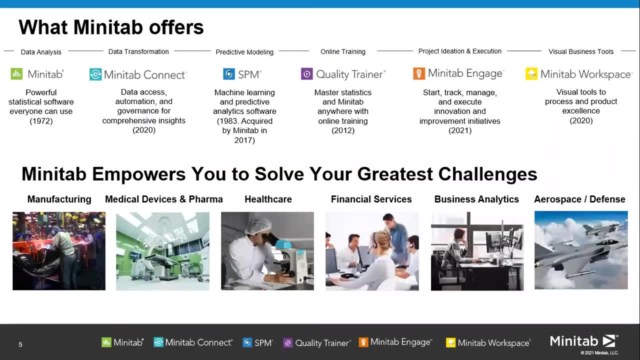 are statistician or non-statistician, or you are data scientist or non-data scientist. So our flagship product is a Minitab statistical software, and we have five other products as well. They are Minitab, connect to transformation and for the dashboard, And then we have a 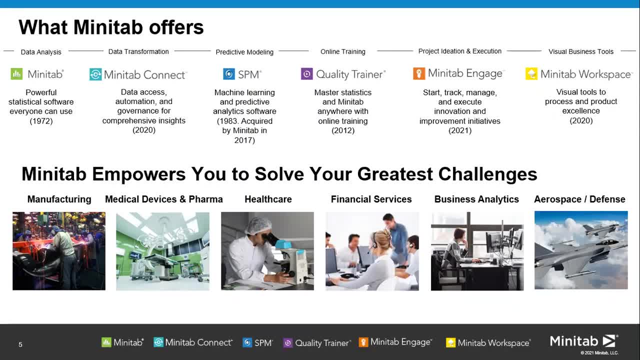 software, predictive modeler for the machine learning and predictive analytics. So, but nowadays some of the algorithms inside the SPN are available. Thank you, Minitab. statistical software. And then we have the quality trainer. The one is the online. training consists of few models like statistical inferences, regression, DOE and so on. And then 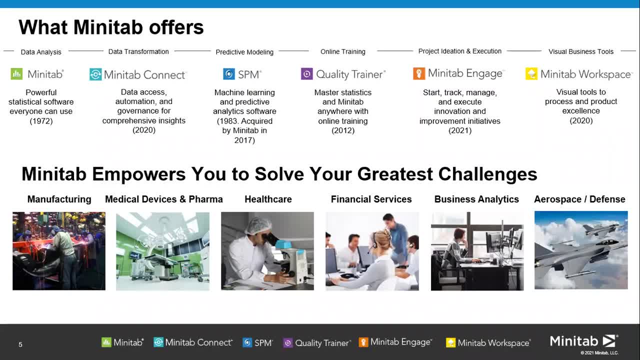 we have a Minitab. engage is for ideation execution project, and then Minitab workspace for visual lifestyle template like VSM, FME and so on. But today we focus on Minitab statistical software With specific tools. it will be design experiment. So if let's say you are interested further, 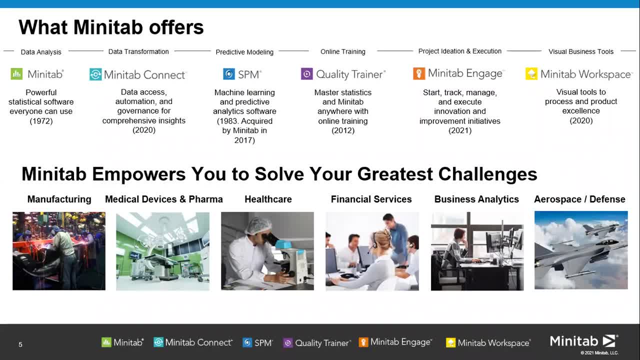 to know other products, let we know. we provide on all the product demo, on offer for all the product. Okay, And then Minitab is will use from many various industry As a manufacturer- I think most of you coming from the manufacturing itself. And then we have a medical device. 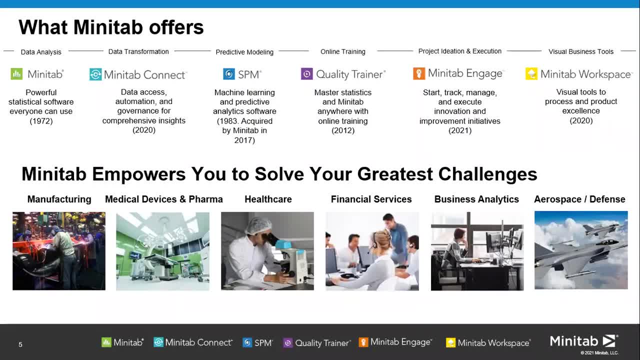 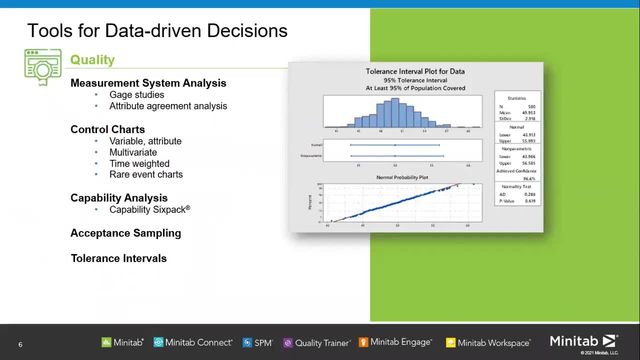 and pharmaceutical customer. We have healthcare customer. also, We have the financial services and so on. And then here is some of the tools available in Minitab statistical software, For example, in a quality site. So we have a measurement system, analysis, And then after that we go further: how to know? 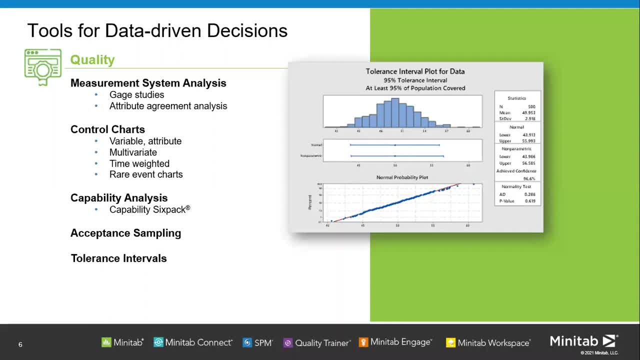 or how to monitor our process with using the control chart. And then we have the capability analysis. Okay, So all these measurement system analysis, control chart and capability analysis- we have already have a webinar on that, So I will share the link for you, For those are. 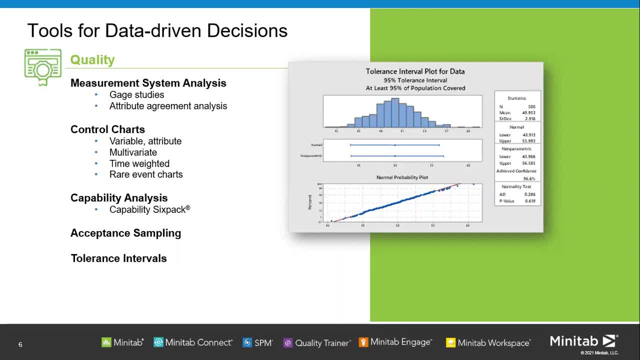 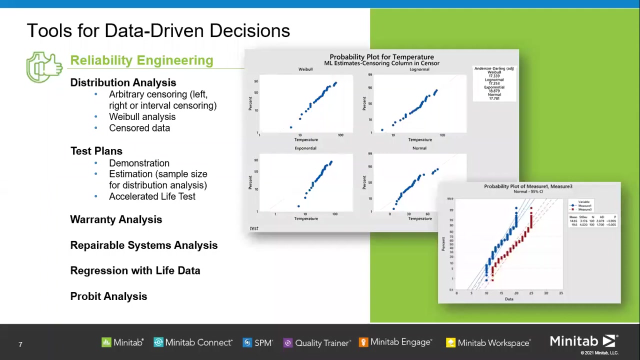 not available to watch to join our previous webinar. regarding the measurement system analysis. we have a control chart and then we have the capability analysis, So I will share this link on the chat box, Okay, And then we have other tools available for the reliability engineering And then for 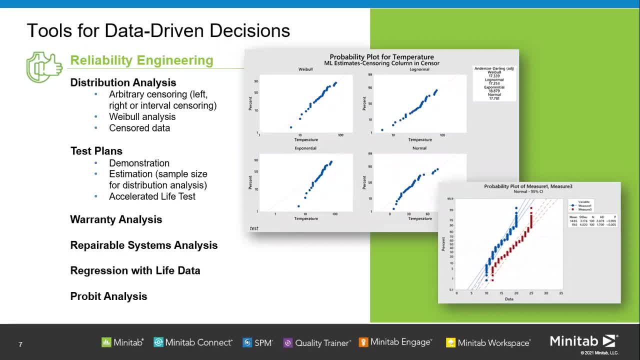 your information. Minitab 21 have a new tool for the reliability We have a cork regression, Okay, And then also we have- today's session is focused on this one for the DOE design software- Okay, And then also we have- today's session is focused on this one for the DOE. 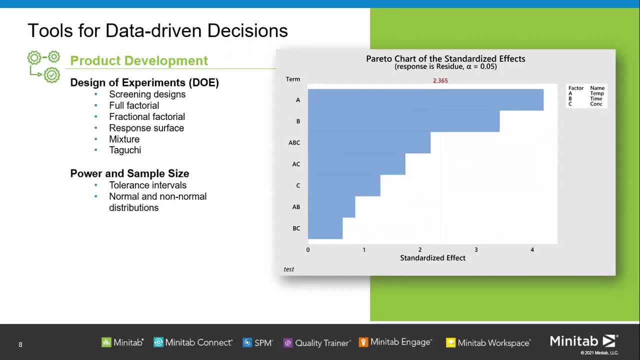 design software: Okay, And then also we have today's session is focused on this one for the DIYT Biz today: Okay, And then also we have today's session is focused on the test design of experiment. so, but today we not only cover all the 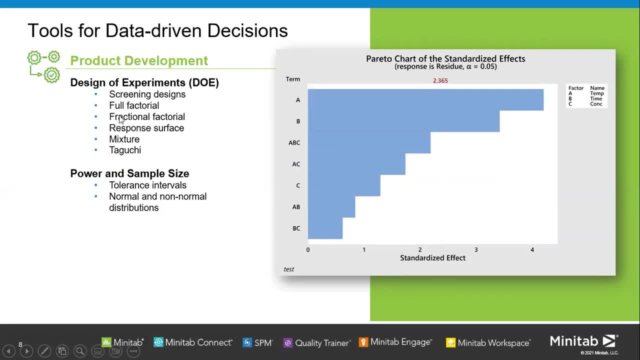 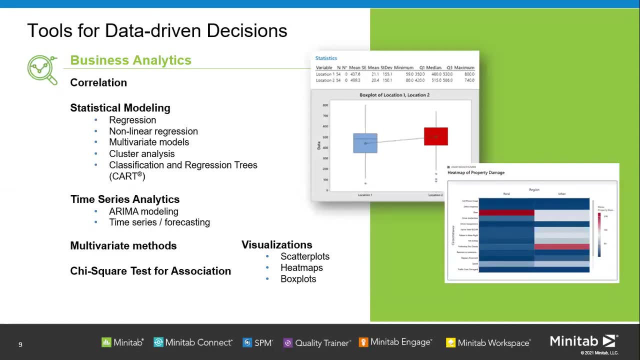 six, design. we focus on the uh full factory design, okay, and then we have also, uh, i just think like business analytic is something like you doesn't have any requirement to do the experimental, but you want to do the prediction, so we're able to have something like uh, statistical. 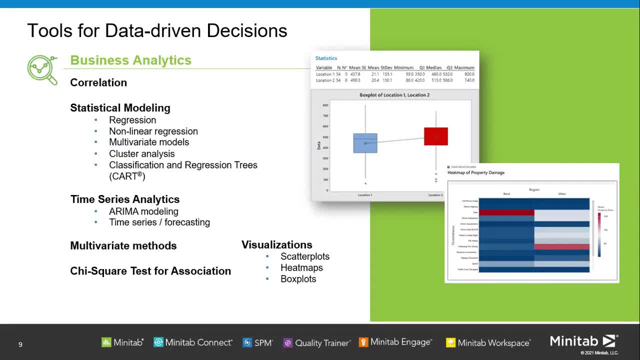 modeling like regression itself. we have the time series itself, we have the multivariate of eternal, easy something that one. and then we just added, instead of missing minute at 19, we have to. we call it classification and regression tree, okay, and then we have the process. uh, 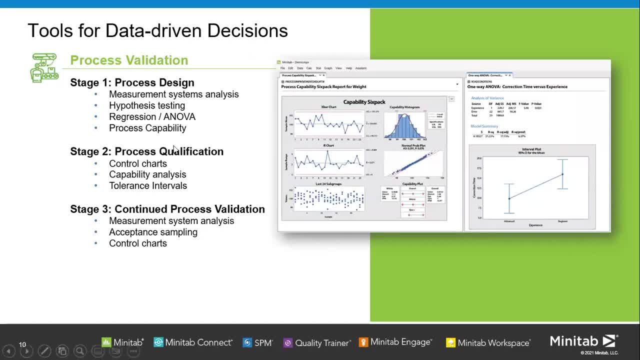 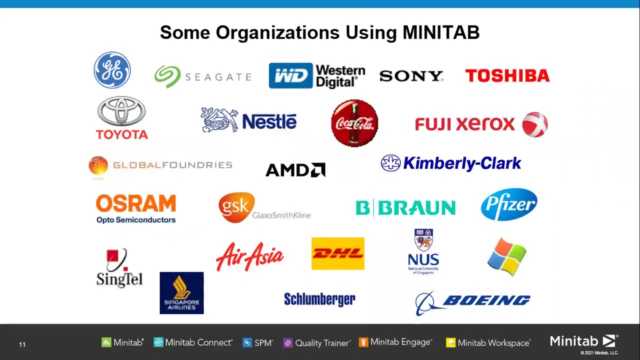 validation. but just i want to highlight here, okay, that one, this uh toast is not like in this sequence. it will be from different uh medium. okay, and then here is the since in the method statistical software we have a complete toast for analysis. so our customer is coming from various uh industry. 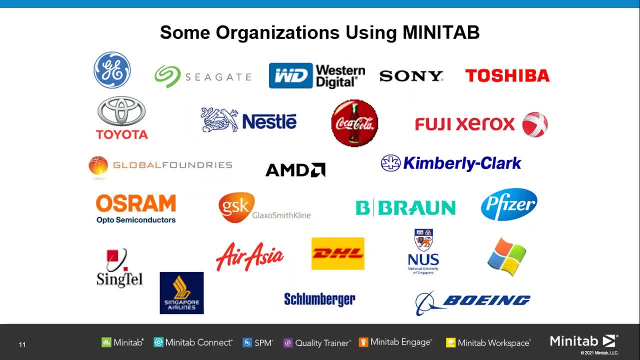 okay, and then all the type of a car company is can maybe can be a multinational company or can be uh from the small, uh sme company also fit to use this software if you your aim to be a data-driven company. so today agenda is related with the. i think it's the most popular. 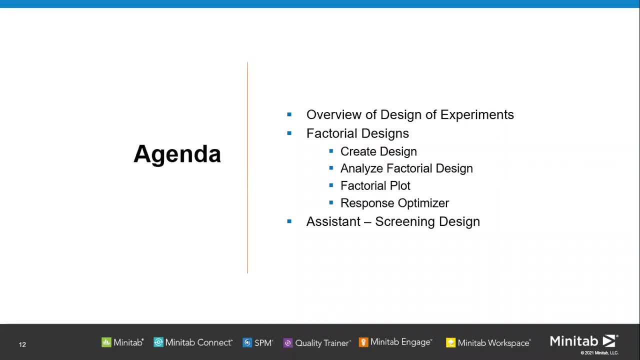 normally used by our customers. it will be design of experiment. so we try today demo. start from the how to create design itself from the mini tab. not only start from basic example model, but like from the data strategy of all models, like the similarity, also from the model language, for example. uh bitteterwer, uhע um miney, the moment i'm traveling to south for school of science today having text files that you need to Draw up here to then make it be. it's the way it could. so, um, there are all versions Voice over the hour over the content, but just complete. one more study is all the time we and um would like to. 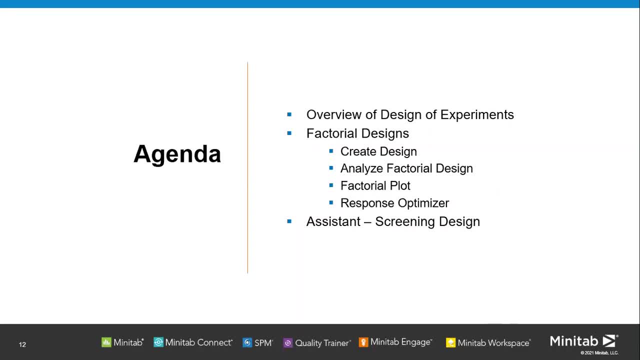 what we be the person's guider. we are going to focus on cost, cost consumption. that's like it's. so i want to start with the analyze: you can create your design itself, and then, after that, you analyze your, your, your experimental, uh, using the statistical, those like anova, regression and so on, and then after 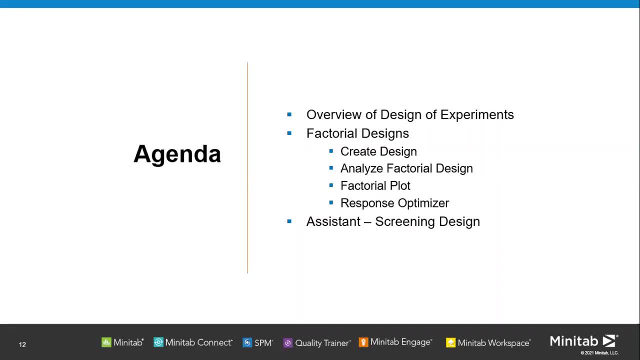 that we go for the optimization, we have a response optimizer and then after that we we try, with the simple snap of the last last step to run the minute. uh, design for experiment using the assistant. i think if, let's say, you are all user of this mini tab, i think you are already know about the assistant. 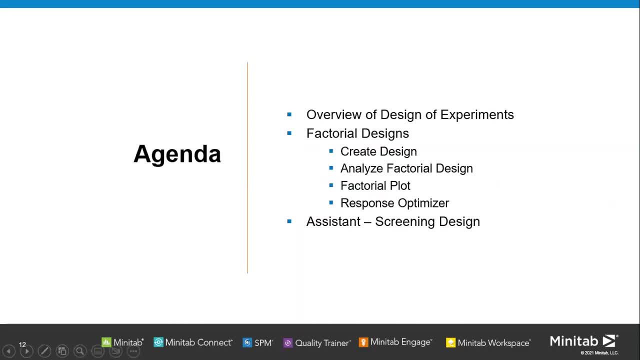 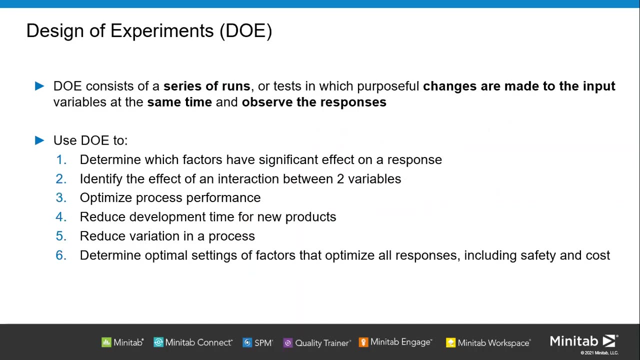 okay, so hopefully, in one hour sharing today, you're able to see how the oe works and maybe the oe will be one of the tools to solve your problem. okay, so the design experiment is a series- okay, it's a series of run or tests in which, purposely, 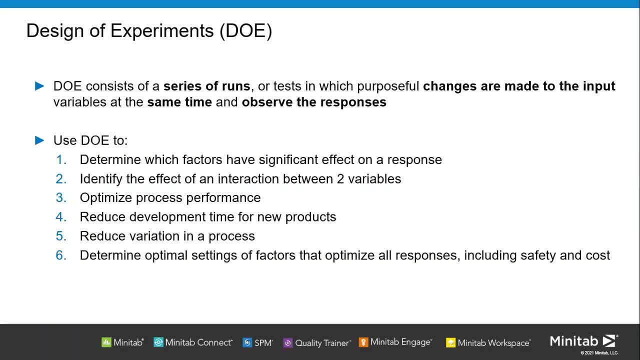 change are made to the input variables at the same time and observe the response. maybe before this in this, in secondary school we already do the experimental. if let's say we took the science subject or something, that one, we already do the experimental. but we mostly we do like something. 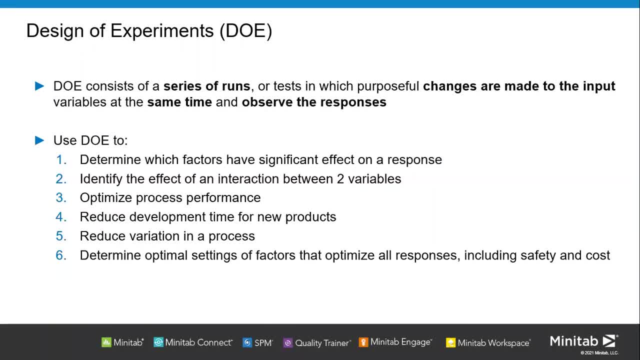 try an error. so we just do on only one time to that, to us ten times and so on. but in them, uh, if you say you're using the experiment design of experiment, they will come up with the- we call it design experiment to know how many runs you should. 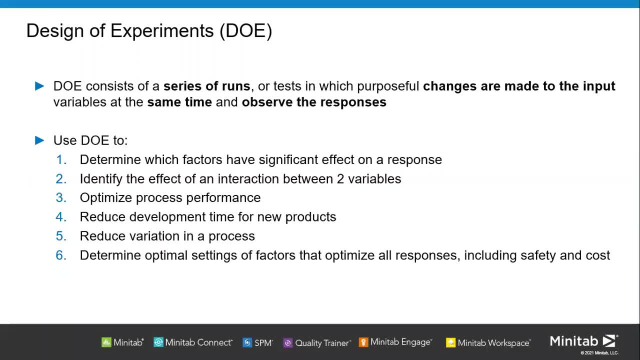 you should do, and then how many repeat detection you need to do, and so on. so that one, that one in design experiment we call that one- is a series of runs- okay, not the only one, maybe it's a combination of your factor and then your level in at the same time. okay. and then in industry, 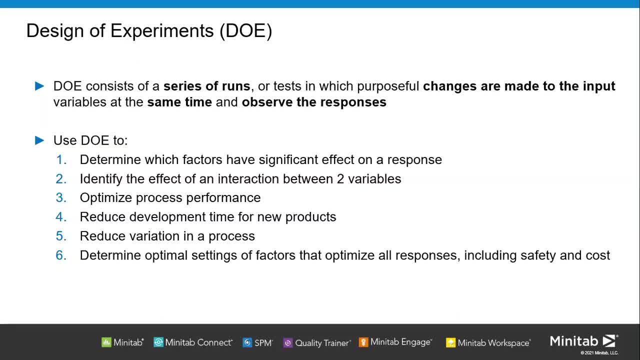 maybe design assessment can be used to systematically investigate the process or product variables that affected the product quality. so for example, just now i mentioned that after you define the process condition like stability and capable, and then you can direct, improve effort to enhance the quality and so on. so DOE here, maybe in the real life after. 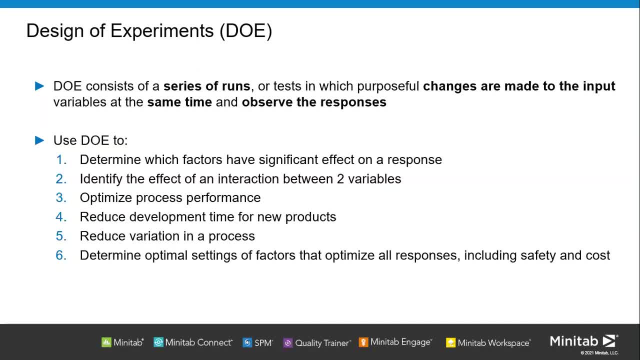 your process is stable and then capable, and then after that you do the DOE. but DOE can be without know about the stability and then without know about the capability, but you might be have some others problem. okay, you will facilitate and then maybe after that you can conclude that DOE is not good way. 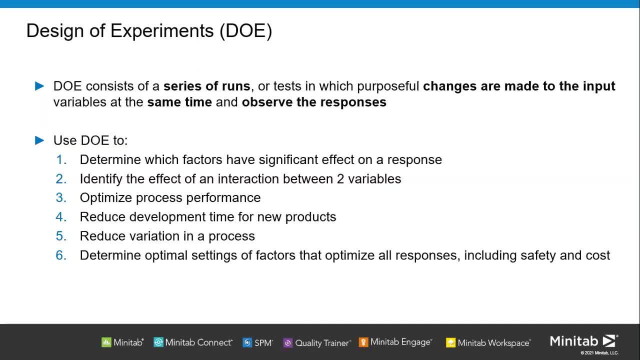 so DOE is something like systematically project or systematically start to run or to do the DOE. so will we use DOE to maybe determine which factor has significant effect on the response itself? maybe you have something like you want to identify the effect of the interaction between two variables and then you want to optimize the 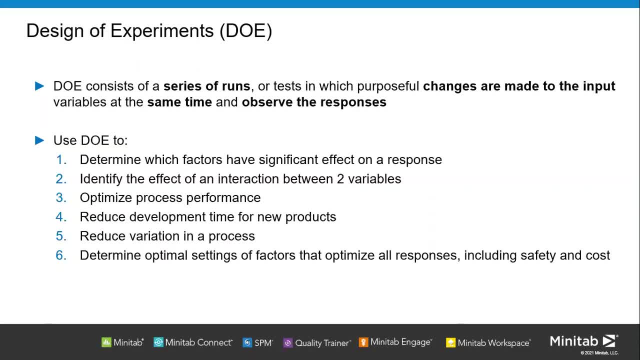 process performance itself. and then you want to reduce development time for the new product- okay, and then you are going to reduce the variation in the process itself. and then, of course, you want to determine the optimal setting of the factor that optimizes all the response. okay, maybe this one is: can one of that you will be, reduce your cost, and so on, okay, 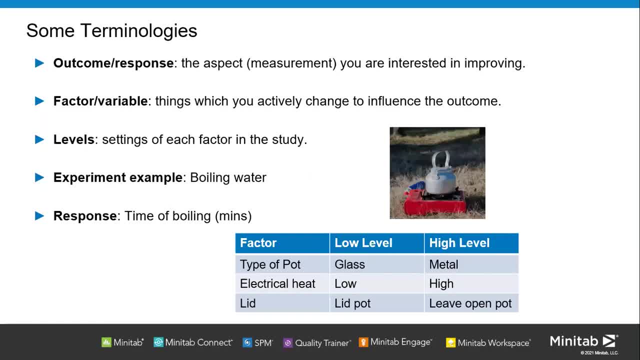 okay, for those are new with the design of experiment isaf, here's some important terminology to know before we go further. the first thing is a response, is a outcome, or come to the mathematics school we call it is a. why is here the aspects measurement- are you interested in improving okay? 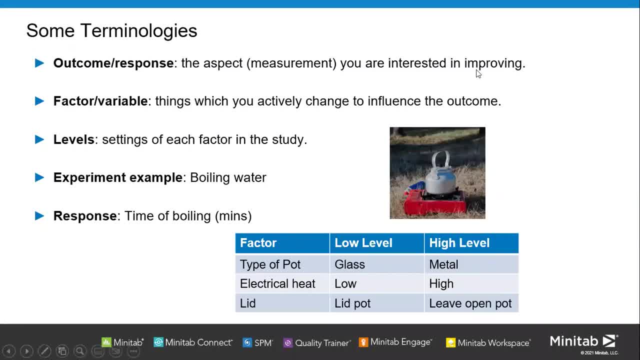 so the term what is here is to improving or something like: uh, for this case, you want to know about the time of boiling. okay, our the critical part, but in term of you in the company, maybe you can go further with the critical to quality, what, what kind of the problem you face it. 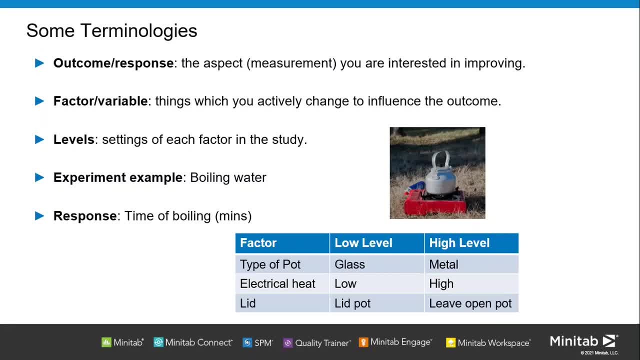 okay, of course you want to increase your satisfaction of your uh customer or something that one. but if you need to convert them into the will be our measurement. and then another term is a. we call it factor, or sometimes we call it variable, or sometimes maybe you will use your parameter, okay. 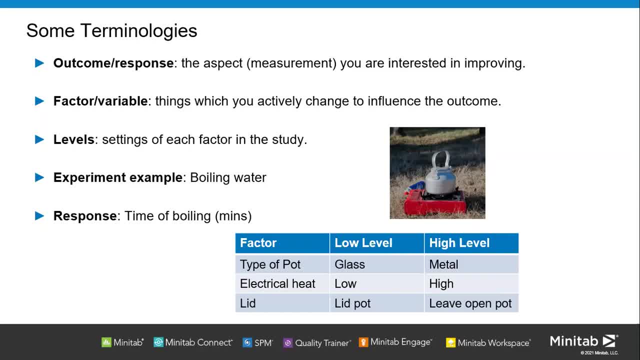 things which you actively change to influence the outcome. and then another thing is the level. is we call it the setting of each factor in the study? for example, here we have a factor of variables. it's a type of part we have electrical heat and then we have to lead, so different is considered the parameter. 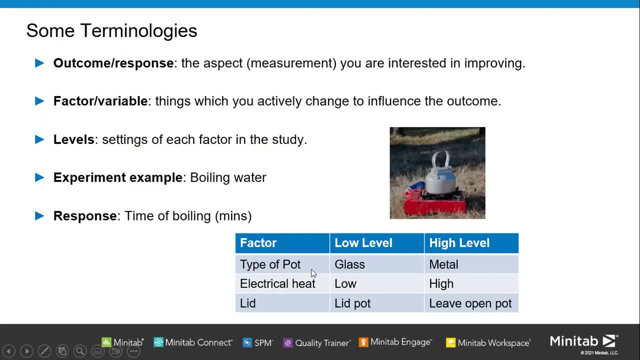 if let's say your type of the pot is something like glass or metal, we consider that one is the level. okay, some, for example, also you want to do the uh, something like. uh, something like baking cake, something that one so and then you go for at the supermarket. you can see a lot of brand. 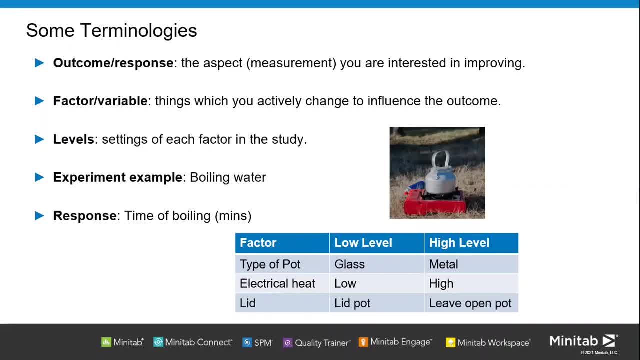 and a lot of type of flow itself, like protein, and then we have the flow normally high, gluten and so on. we have a lot of type of the factor itself. so that's why you want to see which one is the good one. okay, so that one is, you set up the level, we call it. the level can be two, can be more than two. 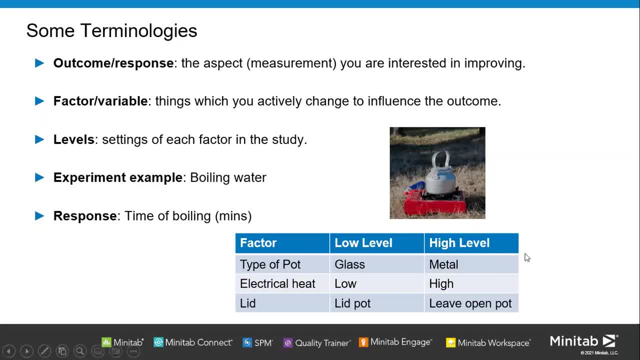 can be three and so on, okay, but if let's say you have more than two, maybe it will be complex for this case. and then we have the experiment example. for this case I want to know about the boiling water and then our response or our outcome is the time of boiling, maybe. 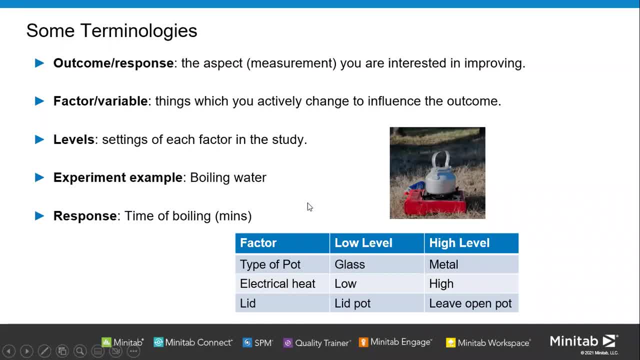 it's a boiling water. maybe you want to know about the structure or the atom: ishf, h2o, something percentage and so on. so so so you can further for this case, but for me i want to just only know about the time of boiling. maybe i. 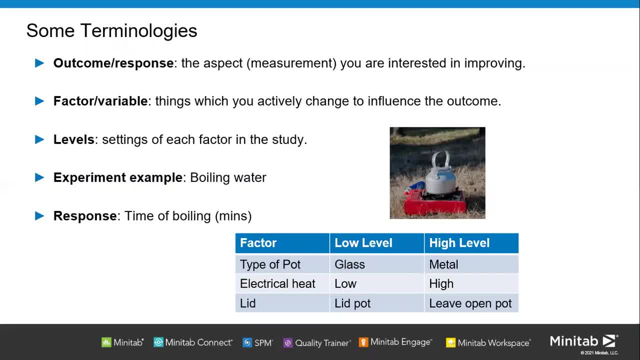 rushing. i just want to uh have a 10 minutes only to prepare all that thing. so i want to last that kind of the number. so that's why maybe i did to do the invest experiment like a type of port i need to using and then i need to look on the electrical heat. maybe i just need to use already for the. 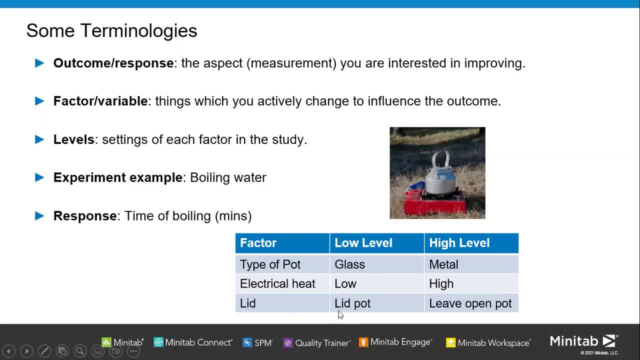 height level, and then i need to have a leap port, so something that one we will try in error, so we not only look on one side. maybe it can be, uh, more than two, better, more than two level, but for, of course, start, we start with the two level. okay, maybe secondary school experimental, we just 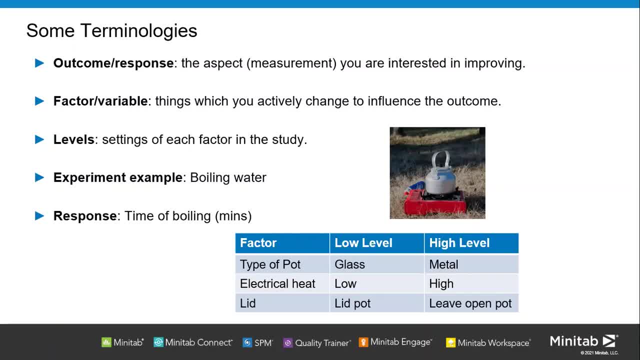 know about the type of part only without setting the level. but now you, in the process itself, in the real life, you want to see more on the level itself. you already know about the factor, but which level, what level you is want to see on this one. so hopefully you will get some terminology here if let's say i say that about. 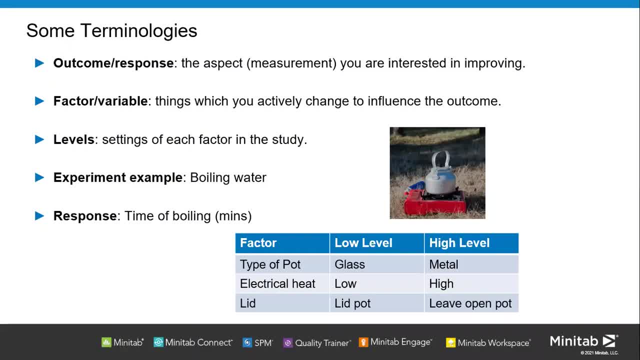 the parameter, how many parameter you have and then how many level you have for each parameter. so of course cannot must be like same level. no, if let's say, this parameter is a two level, and then we have the two level, so we have the three level, so we'll we have for kind of the design itself. okay, not not. 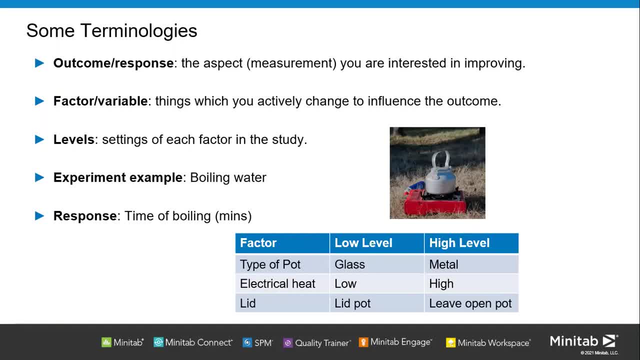 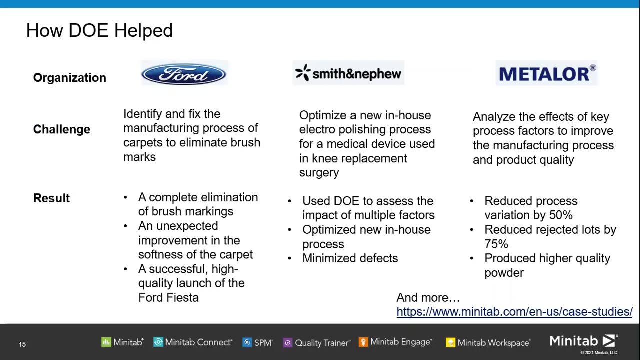 we call it the factorial. maybe we are this name for the. we call it the mixture design, so more complex on this one. okay, so let we go. so if let's say you want to more about the success story, uh, about the doe, the, our customers already uh run or a payment in their company, so you want to have the. 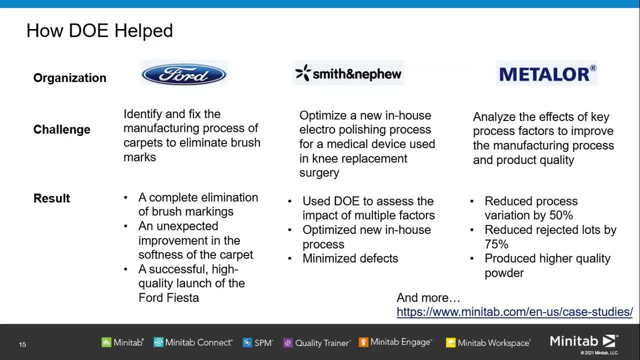 success story uh about the doe the. our customers already uh run or a payment in their company. so you are able to see in this our case study. okay, so i will uh share the links, how to get it, how you can get the success story. okay, so after the 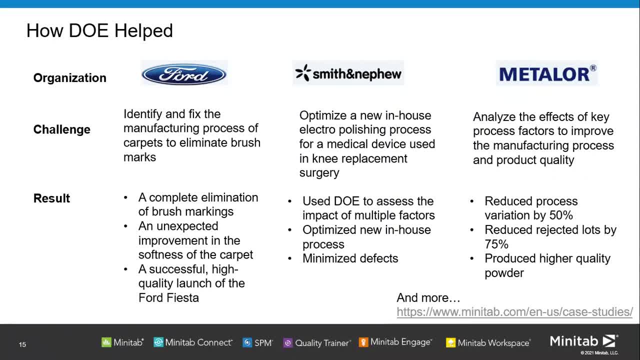 okay, i will just pass uh paste this link to. okay, so i will just pass uh paste this link to the chat pop. okay, so you will be able after these. if let's andy, you will be able after these. if let's say you have a time, so you, maybe you have possible after this if i say you have a time, so you. 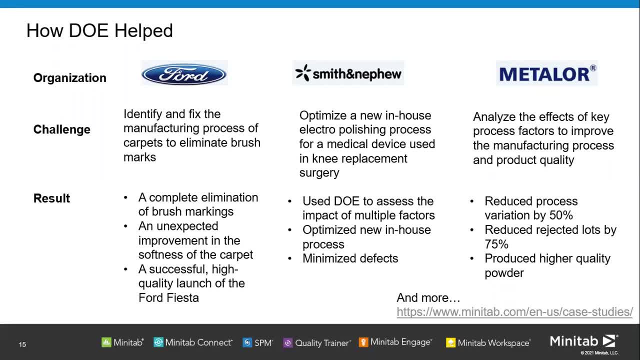 So you can see the other successful story about the Minitab and then about the specific about the DOE itself. So DOE is not only for MNSC company, SME company also can do the Minitab okay. So if let's say you have a challenge or you have problem, like want to identify the fixed manufacturing process, 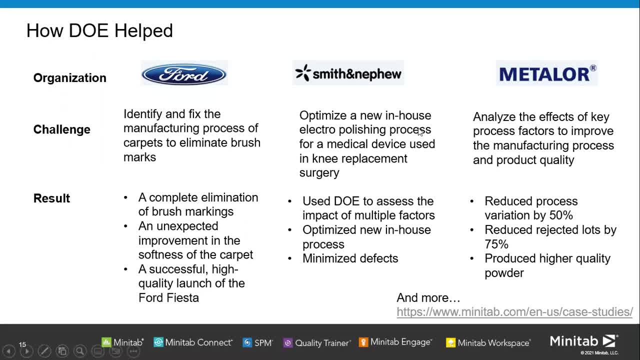 something that one from the fault itself. or maybe you want to optimize a new in-house electro polishing process, or you want to analyze the effect of the key process factor to improve the manufacturing process. So all these kind of the problem you face it. maybe you will be proceed with the DOE, okay. 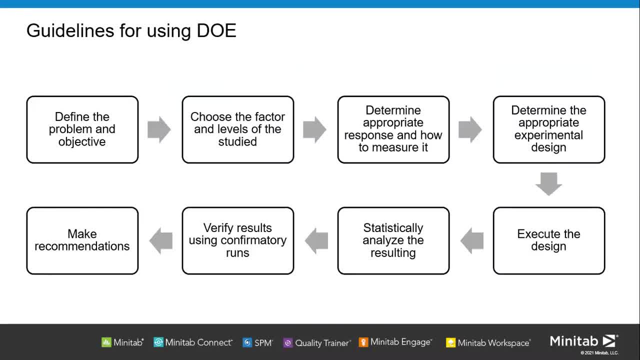 So here is some guidelines to run the DOE. okay, Of course, this is the first three steps. here is that you find the project and then you choose the factor and the level, and then you determine the process, the response and how to measure it. 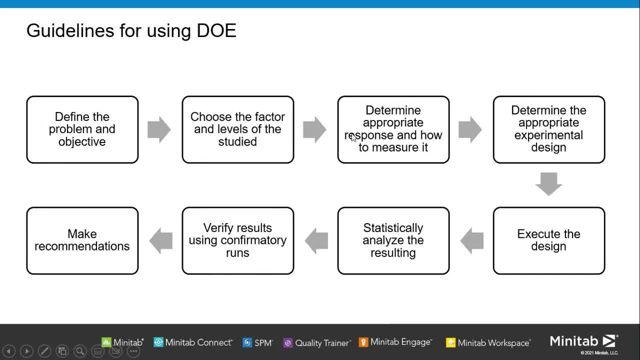 So all these three steps I think most of you already know. okay, If, let's say, you go for the specific part, also you need to have the problem problem statement and so on. So after the differences between the other project with this DOE, as we call it, this one. 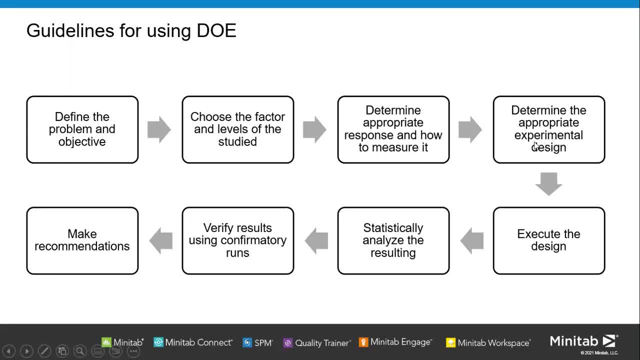 it's experimental, Okay. so to decide which type of the experimental design you need to use, it will depends on how many factor you decide and how many level you decide. Of course, it will be related with your costing and your time, okay. 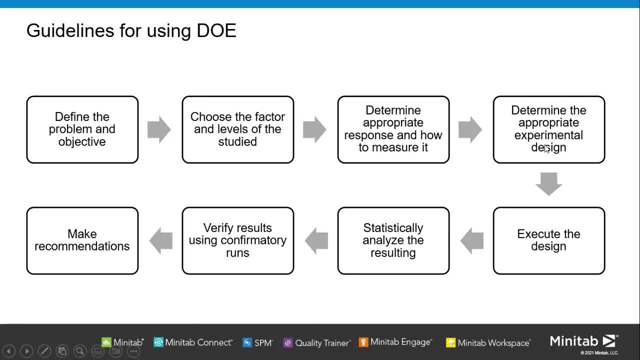 And then after you decide what type of design you should do, okay, And then now you know how many, what type of design you must run. Okay, for example, you have a two-factor, two-level, So two power of two, which is is a four run. 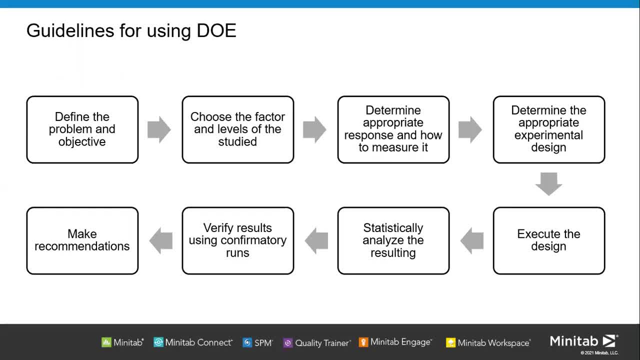 Okay, two power of two is a four run, So for run only one replicate. if let's say you want to more accurate, maybe you can go for the three replications. So four times with the three. So need to run about the 12th run experiment. 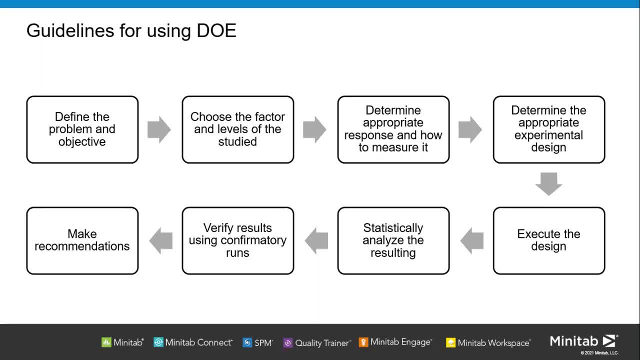 So maybe one experiment, So four times with the three So need to run about the 12th run experiment will cost how many and then how many duration you need to take for one run. So from here, from the experimental design, you will know how many run you need to run and so on. 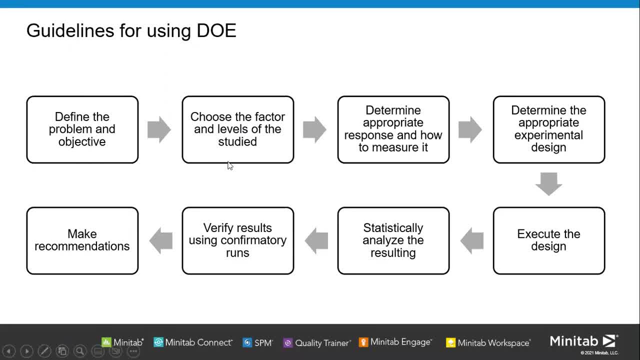 It will depend on how many factors you decide, how many levels you decide. After that you can run the analysis based on the design itself And then after that you can proceed with the others, with the statistical analysis like ANOVA, like regression. 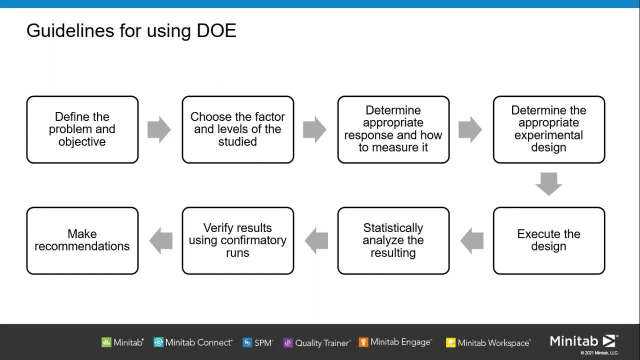 And then maybe you can go to visualize something like using the factor real plot, cube plot and so on. So you have to confirm the result and then you will use it And then you will make it as a recommendation from your design process. 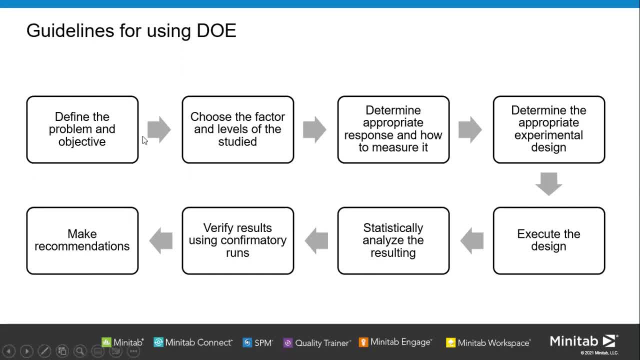 So design experiment is something like it's not stop after finish you stop. No, it's something like continuity. So that's why DOE will be on one of the tools inside the continuity project or improvement project. So it will be some. you have a new problem, so it can be like this one. 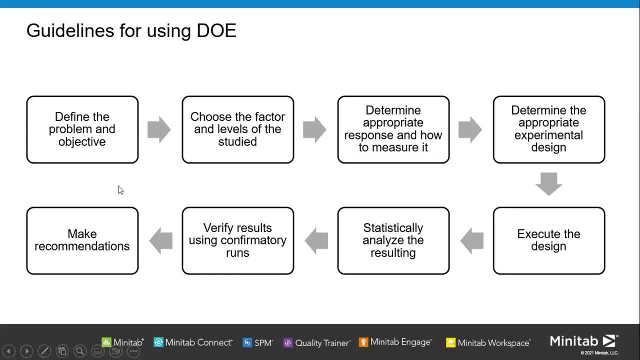 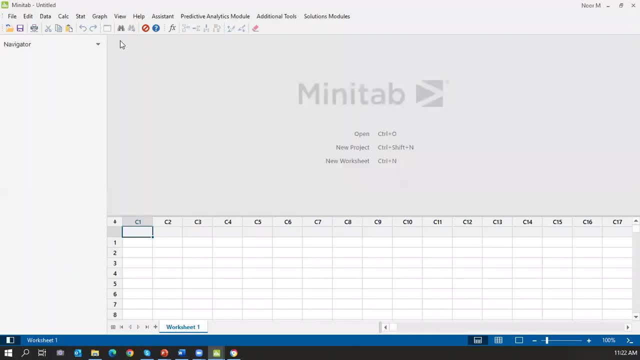 And then you have come in with the new problem. you can build it like the best. And then the- I'm not sure you are Familiar or not, this one, so I will show in the Minitab. So if, let's say, you open the Minitab, actually the step will Minitab will show for you. 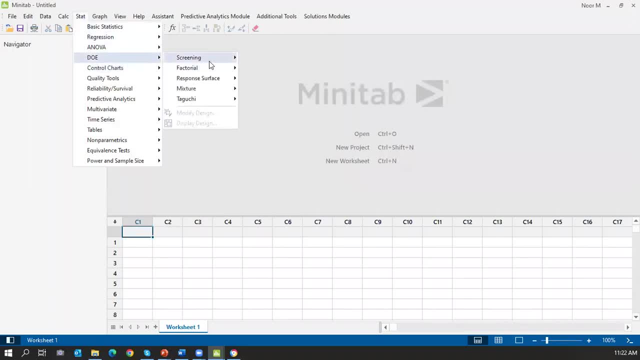 So you can go for the step, go for the DOE, and then you can see the factor, for example: Okay, you can see the create. You must create the design first And then in the gray here, so you can see that you cannot. 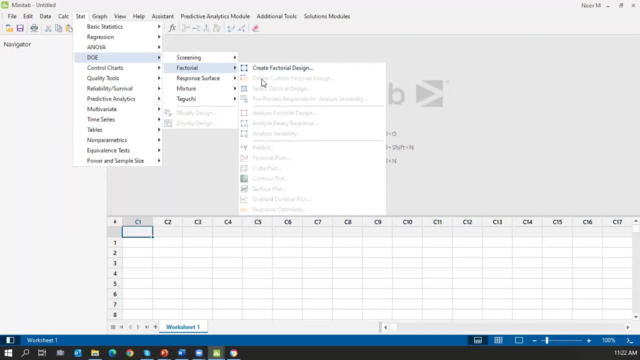 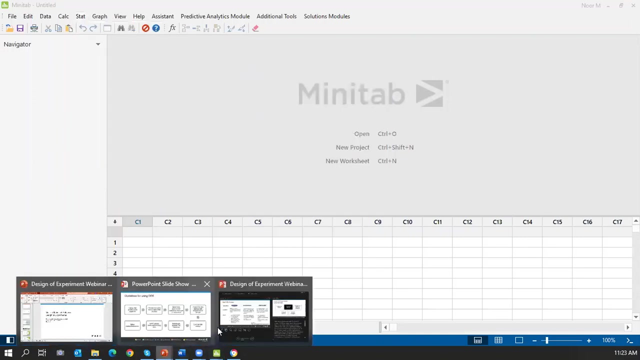 Okay, Minitab will give you some idea. So meaning that you need to finish the Okay Or create the design first Before you can further for analyze, you can further for predict, you can further for respond optimizer. So if let's say, we look back on this one, so it will be the same. 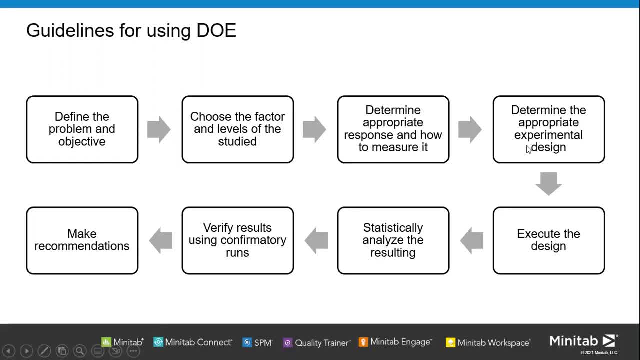 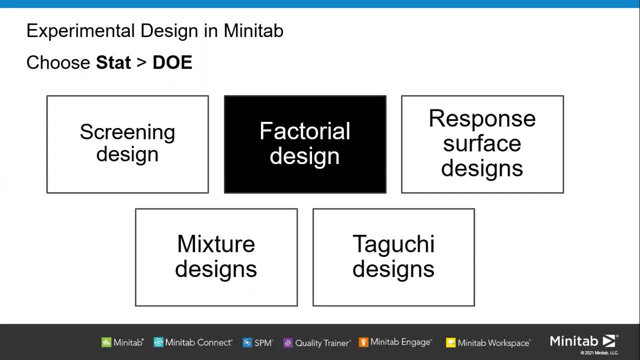 Okay, So you are able to see this guideline in the Minitab statistical software. Okay, So Minitab offer the following design experiment. For example, it's a screening design. We have the factorial design, we have the response surface design, we have mixture design, we have the Taguchi design. 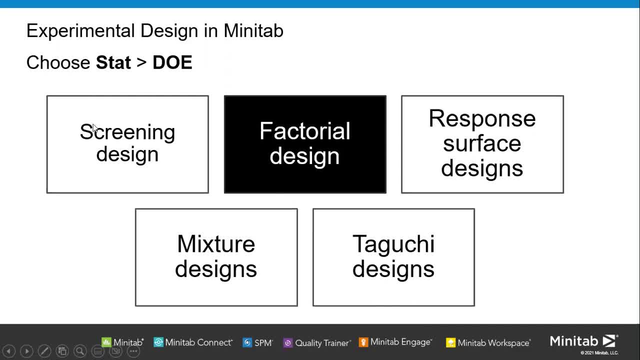 But today I will focus on the factorial design For your information, screening design may be for the starting with the experimental. You have a lot type of the factor, maybe more than 10 factor you have, So you might be go for the screening design. 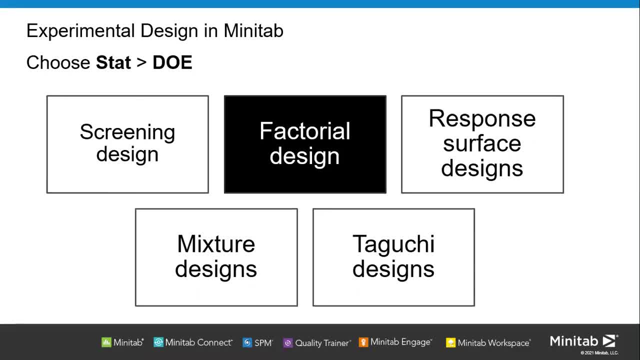 After you screen the design maybe only have five factors With the two level, maybe you can go for the factorial design. So inside the factorial design we have full factorial design, We have fractional factorial design and so on. But if, let's say, your response itself has something like curvature, it's something not straight line. 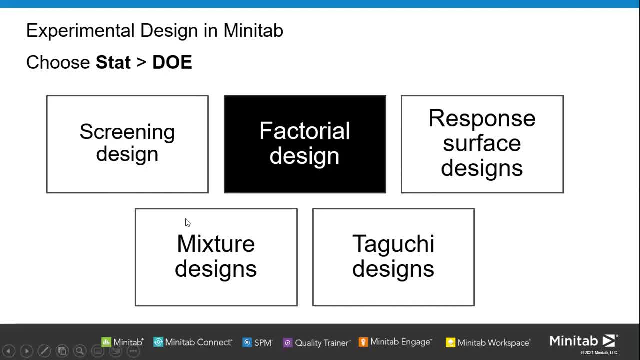 So you can go for the response: surface design. So if let's say your design, your factor, have the mixed level and then you can go for the mixed design, Maybe you won't look on the loss of function, something that one is. you consider the noise. 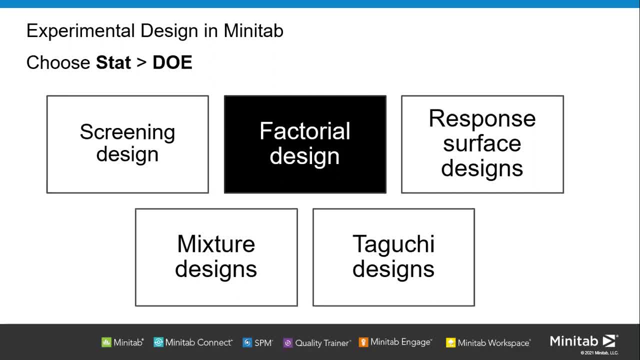 Maybe you can see on your experimental, maybe you can go for the Taguchi design. So this one is a level in Minitab. So how to get it, How to get this one, So you could go for the start, go for DOE. 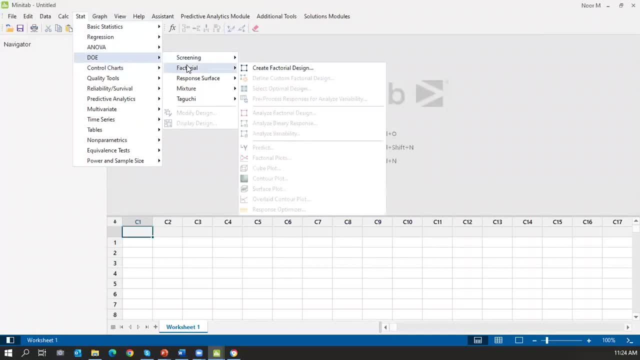 Okay, So you can see that screening side. we have the factorial, we have the response surface, we have the mixture and then we have the Taguchi. So for those are new, with the Minitab, Starting with the Minitab 19.. 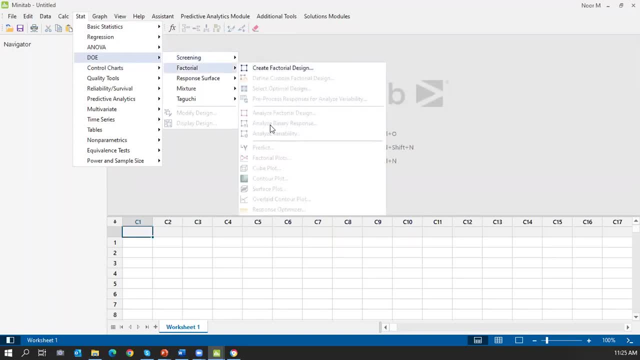 Minitab already have a put another way, We call it the analyzed binary response. So for information, your response can be categorical or can be binary, Something like yes or no, Something that one the text can be for the response, Not only the measurement, like measuring like weight, height and so on. 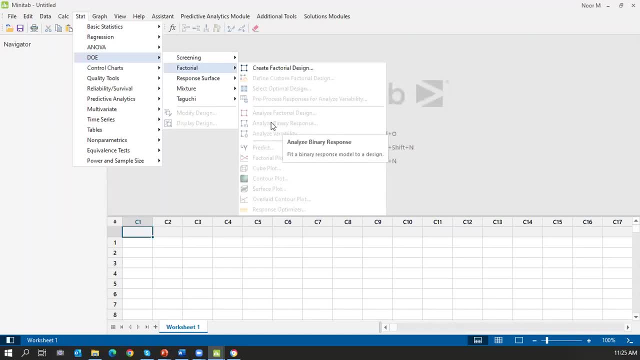 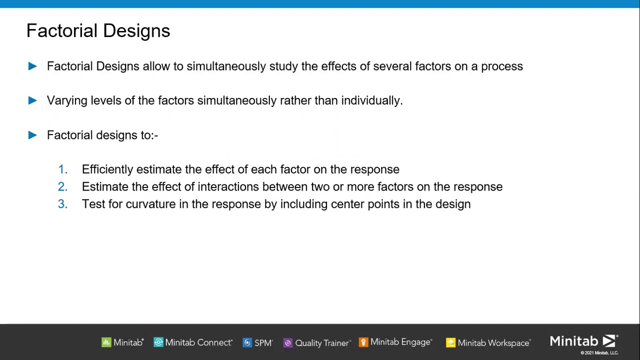 So maybe you can have something like accept or reject, because we have a analyzed binary response for this case. Okay, So what is mean by factorial design? So factorial design allow to simultaneously study of the effect of several factor and on a process, So varying level of the factor simultaneously rather than individually. 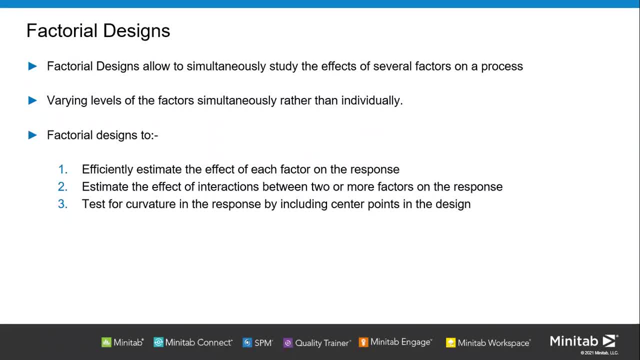 So in the factorial design itself, we combine all. the level We look for, For example, is a temperature: Okay, We have a temperature 20.. We have temperature 40, something that one, And then you combine in this one one trial. 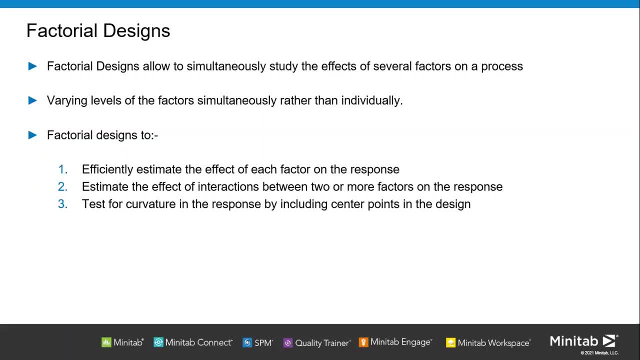 Okay, We can have a temperature with the 20 and then the duration of five maybe can be at 10 minutes. Okay, Next, next experimental, next trial. maybe temperature can be 50,, 40. And then the time or the duration can be 20,, something that one is a combination. 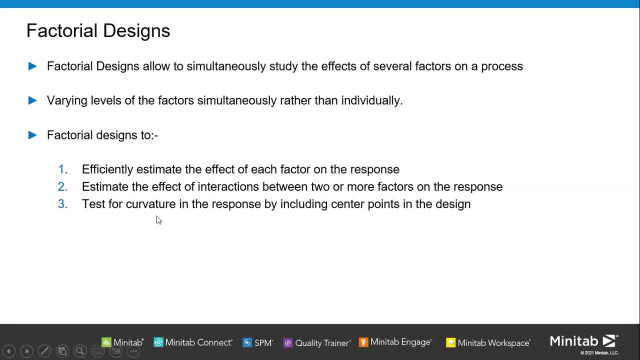 And then for your information, factorial design is to efficiently estimate the effect of each factor on the response itself, Estimate the effect of interaction between the two or more factor and then test the curvature in the response by including the center point in the design. This one is something like a height. 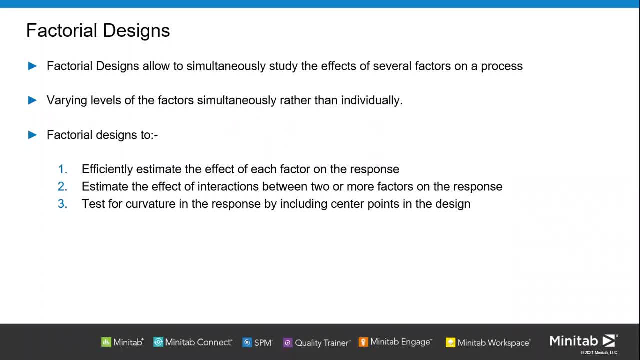 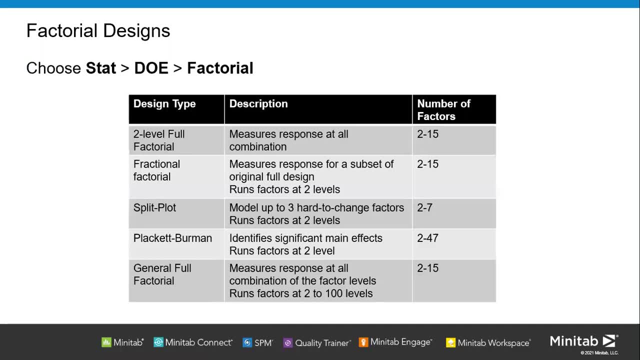 Okay, It's a curvature, It's just not Okay, Only straight line, maybe uh, maybe uh, QB or maybe quadratic and so on. Okay, It's more more technically. So for the for today's design, we have a design type, something like we call it. 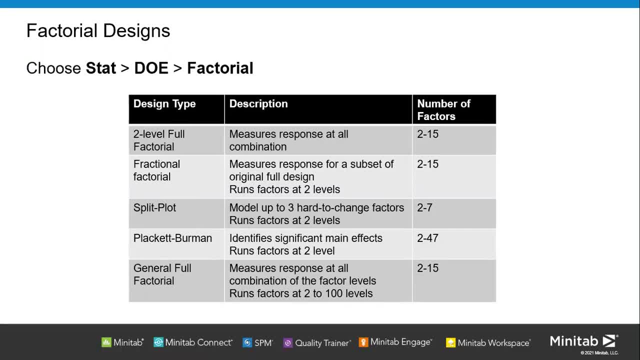 If let's say: you see, or you Google, is a full factor design Okay, So it can be in well factor design, Okay, And then we have a fractional factorial design, and then we have split plot and we have uh, uh, boomer. 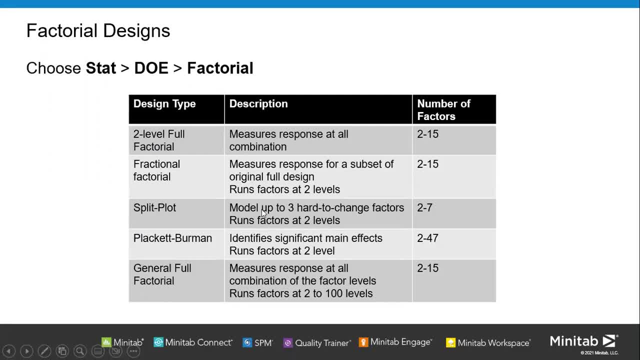 And then we have general full factorial. So even if that they will give you guideline, if let's say, you measure all the combination and then the number of your factor is two up to one, five, So you can go for the two level factorial. 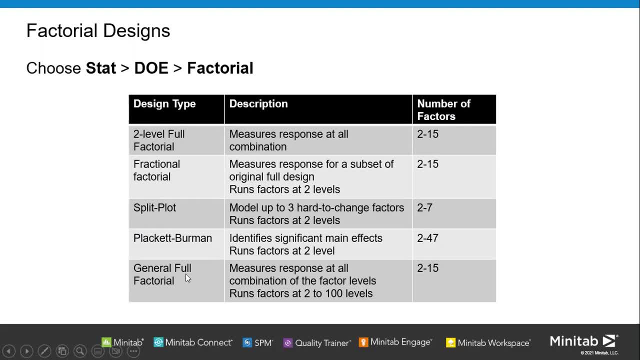 Okay If let's say you have not the two level, but maybe you can go for directly to the general full factorial. If let's say you want to see on the half factorial, okay, Half factorial, So you can go for the fractional factorial. 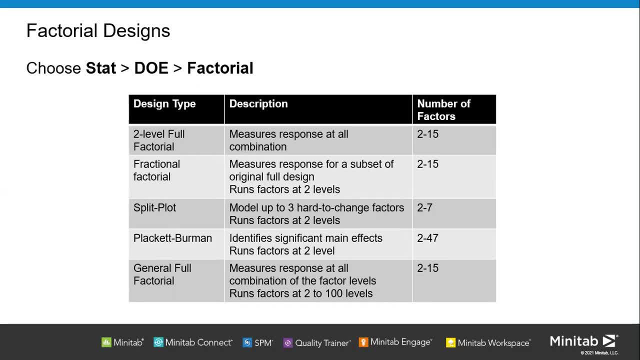 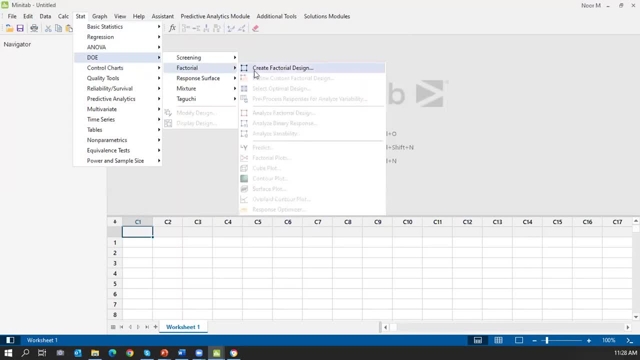 So I will show. So you go back to the, we go back to the mini tab. Okay, Go back to the mini tab. You go for the step, you go for the DOE factorial design. So you click the create factorial design. 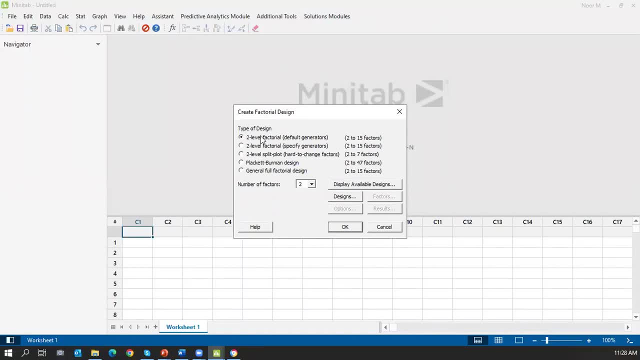 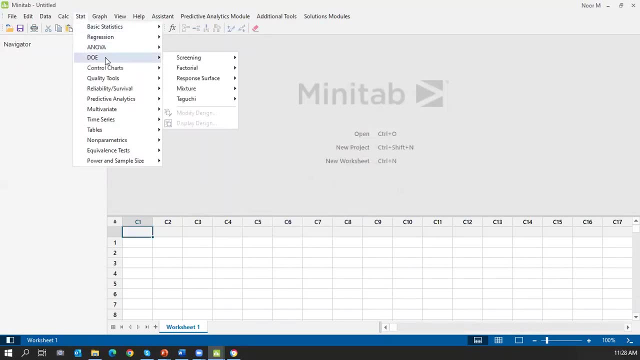 So in here we have a type of the factorial design. Okay, So you, you must clear part: is it for the design itself, design experimental design in mini tab. We have a fact Five. Okay, Design experimental in the factor design. 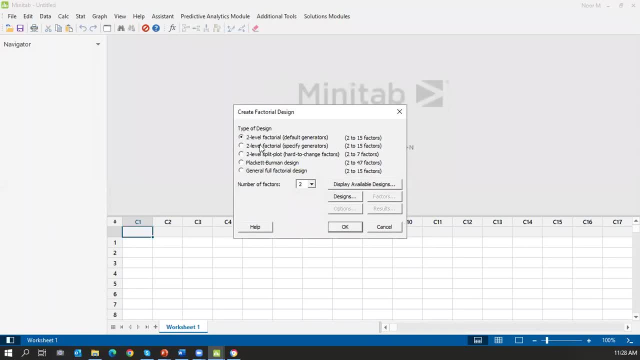 We have type of design. We have two level. We have a two level factorial. We have two level split plot. We have bucket movement. We have the general full factorial design. Okay, And then we go back to this one. Okay. 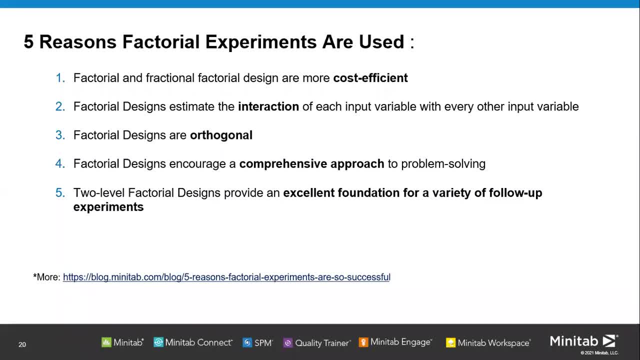 So this one is a five reason why the factorial experiment we use: Okay, The fact factor and fractional design are most cost efficiency, Okay. And then factorial design: estimate the interaction between input variables and every output, uh, other input variables, So we can know about the interaction. and then factorial design are autogonal design. 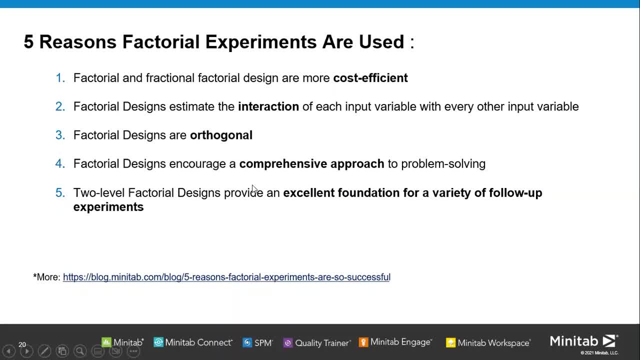 It's a balanced one. And then for the factorial design, encourage to comprehensive approach to problem solving. And then we have a two level factorial, Provide the excellent Foundation for our variety of follow up experiment. So most of the beginner, okay, Most of the researcher, will start with the two level factorial design before we go further for complex one like uh, uh, uh, the Gucci and so on. 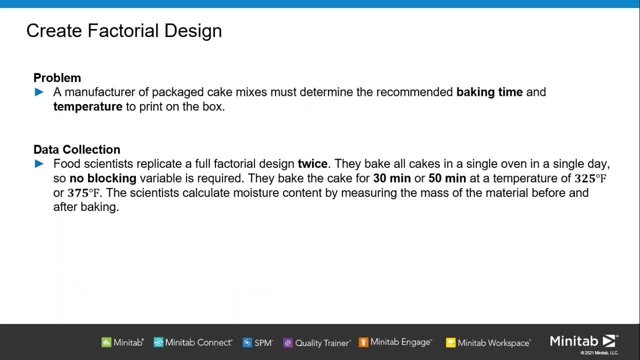 Okay, So we try with this one case study here. a manufacturing uh of packet uh cake mix uh must determine and recommended Backing Time and the temperature to paint on the back on the box. Okay, So for this case, for the food scientists, replicate, replicate uh full factor design twice. 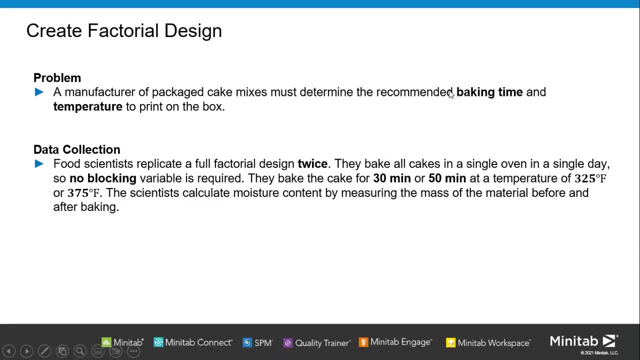 So mean that they provide two factor is a backing, time and temperature. and then they want to use two replication, and then they bake all the uh cake with a single day, So they consider that it's a no blocking, Okay. And then the big, the big uh, the big uh, they bake the cake for 30 minutes and 50 minutes. 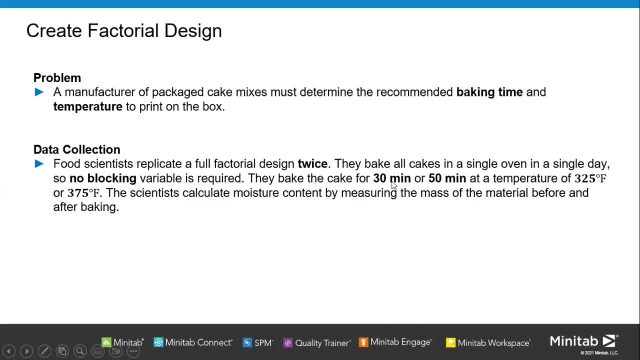 Okay, So back in time here. they provide two level: first is a 30 minutes and then second one. maybe high level will be 50 minutes And then the temperature here at the three to five Farah height and three seven five. 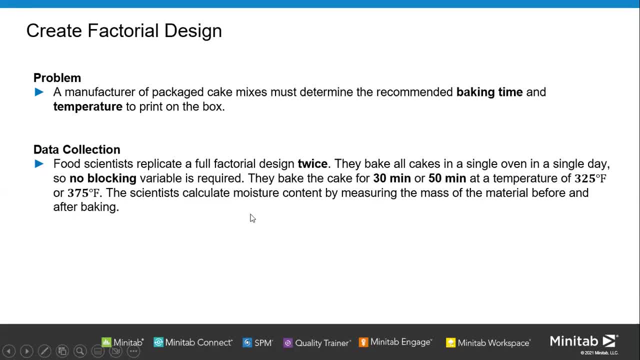 Parah height. And then the scientists calculate the mature content by measure, Okay, The mass of the material before, after baking. So they will measure the why. your response is, uh, moisture, Okay. So for this case they, we have a two factor with the two level. 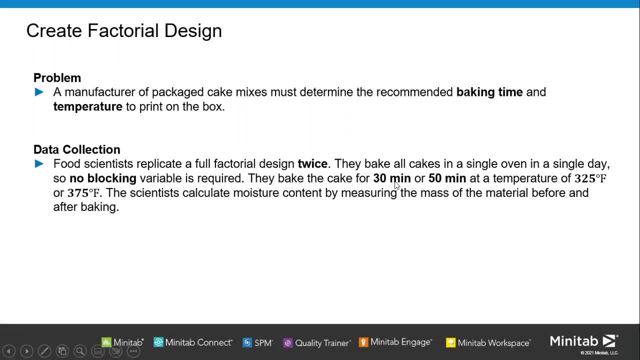 Okay, So every factor have the same uh number of level if we call it the two. So for this case maybe we call it two, two or we call it with a full factory design with the two replication. So how to create the? 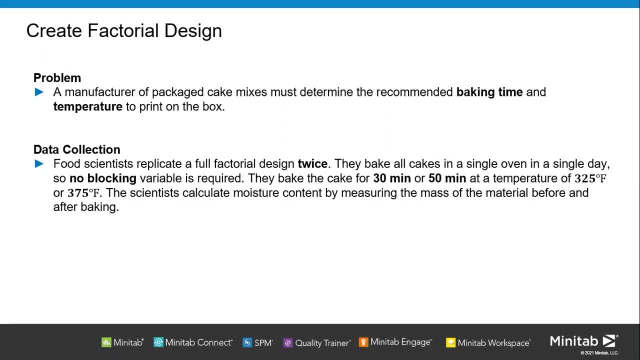 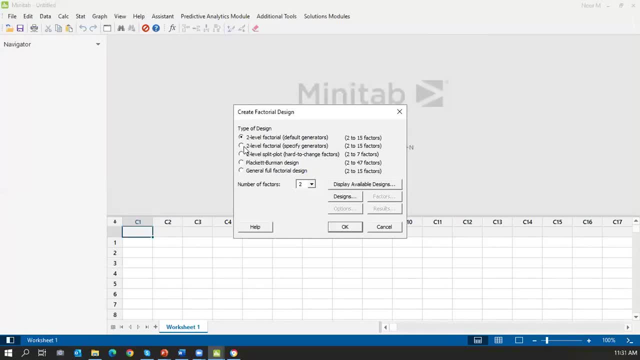 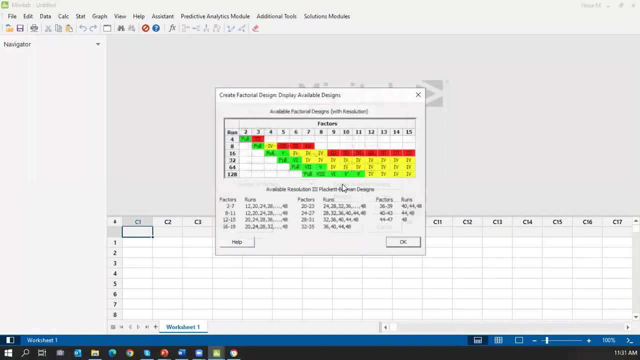 Design itself. So we'll go back to the mini tab. Okay, We go back to the mini tab. So for this case we have a two level: factorial, Okay, And then I will factor is a two up to 50.. So maybe you can go for the display available design. 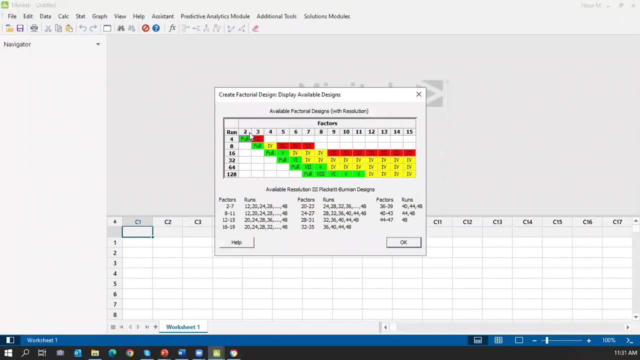 So you can see here, if, let's say, you have a factor, two factor, you choose the full factorial, So mean that your run will be for run. Okay, This one is a we don't Okay. Okay, We don't. 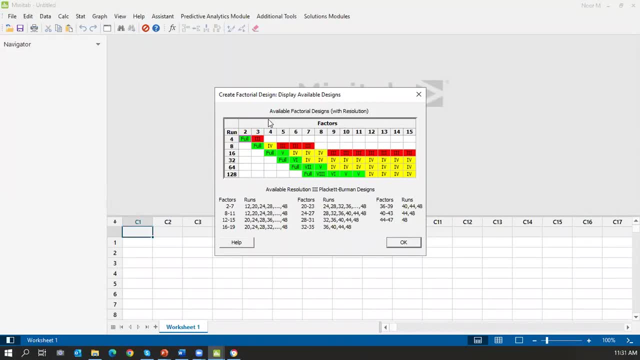 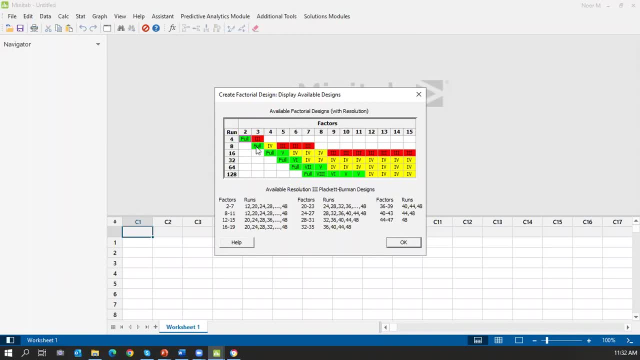 But if I say you want to see more, Okay, You can go for the full. So mean that means to say that is a tool power off three. So how many run you should do is at least eight run, If, let's say, you. 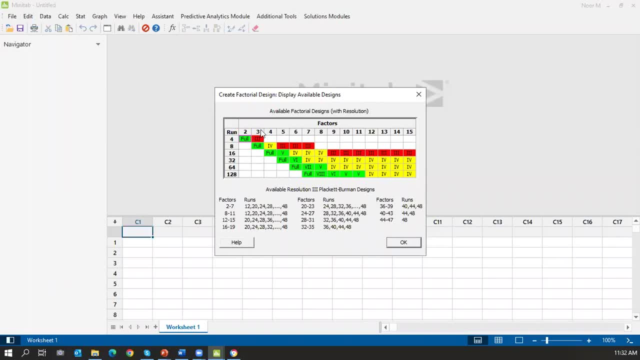 you will see, the 8-run is the most costly. maybe you can go for the 3rd resolution. It only consists of the 4 runs, and so on. So you can see that we have a full factorial, we have the 3rd resolution, and so on. 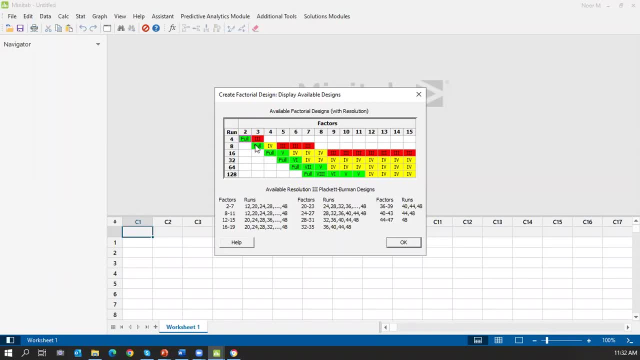 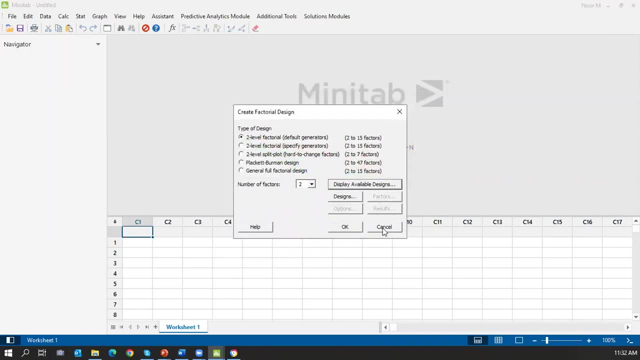 So it will depend on you how many, what type of design you want. For this case I will try with the full factorial and then click OK. This will mean that every time without replication, you must run 4 prior and then go for the design itself. 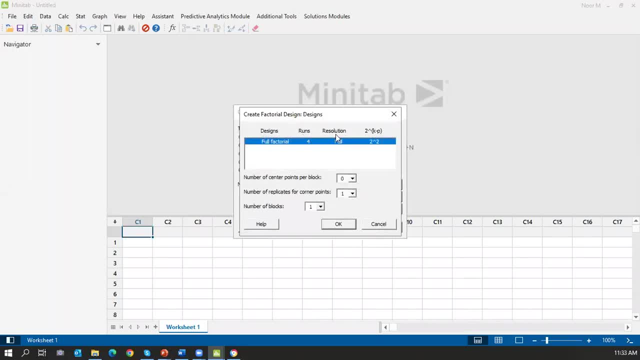 So full factorial with the 4 runs, resolution full. and then this one is a 2 power of 2,, 2 level 2 factor. So for this case, no center point or block, and then the number of replicates is a 2.. 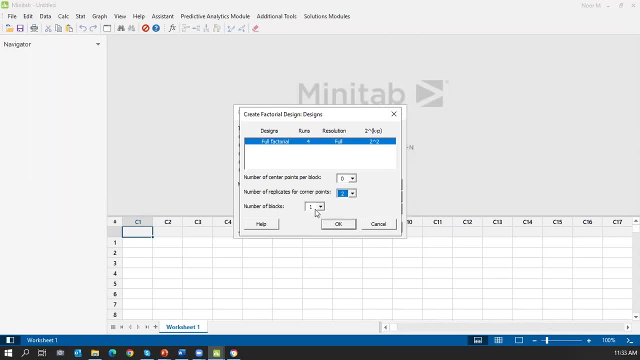 And then the number of blocks is a 0 because they just consider only one day OK, and then click OK. Maybe you, you, you have something like: today you do 5 replicates, another day, another replicate. So maybe you consider that is a half a block. 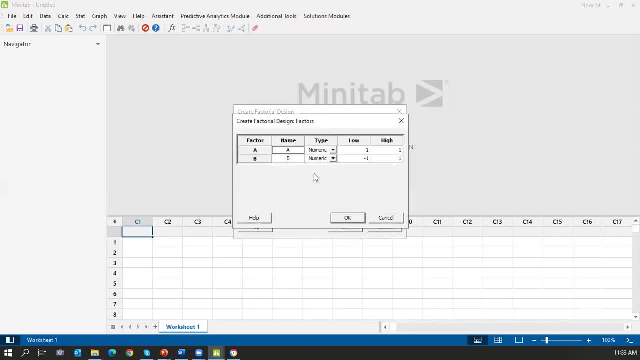 OK, and then you click OK. After that you can go for the factor. For this case maybe factor A is a baking time- OK, baking time. And then the type of this one, the T is measurement, OK, so if let's say categorical can be categorical. 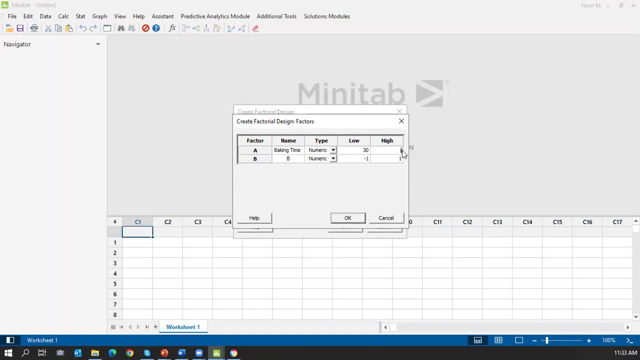 OK, and here is 30 minutes, Here is 50 minutes. OK, so here is the temperature. OK, so here is: the lower level is a 3 to 5, height level is a 375.. OK, and then you click OK. 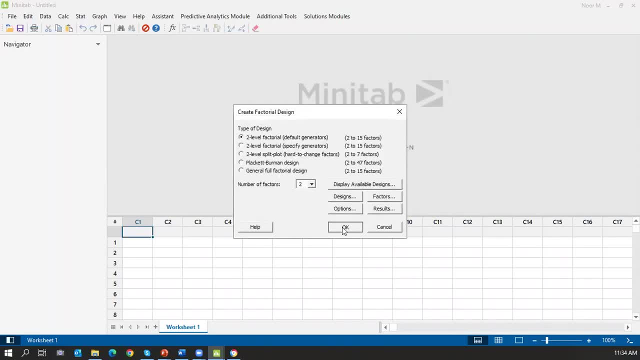 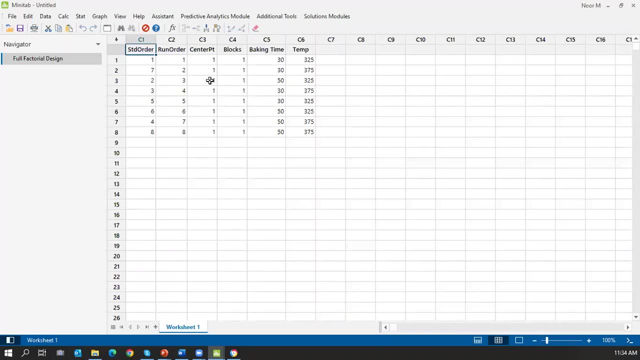 So if let's say you have more than so you can set more than then, you click OK. So now they will appear, We call it. this one is a design, So how to read it, How to prepare it. So the first trial here, the first run here, your combination should be several times. 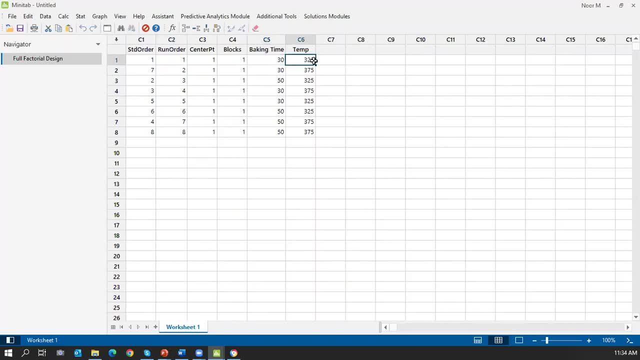 30 minutes and then your temperature 3 to 5.. So your y here is the most sugar, how many before and after You get the value? here, for example, it's 50, something like wallah. And then the second run you should be is combination this baking time and 30, and then temperature. 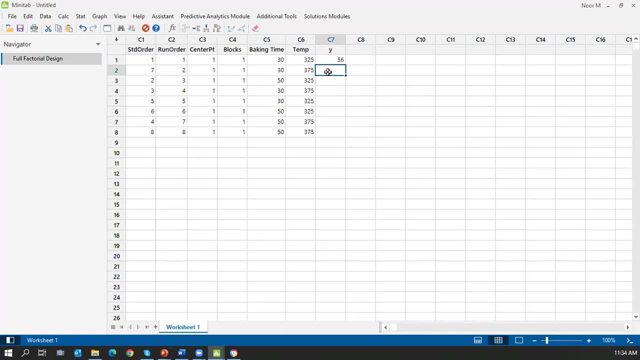 at 7, 48 minutes 35. So we will do the second run and so on. So because this one has two replicates, that's why you have an 8 order. This one is standard order, This one is a. 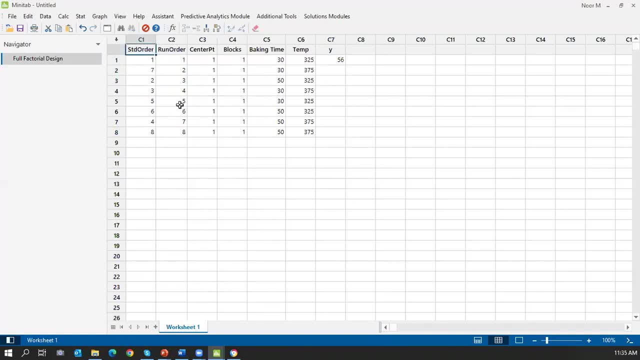 run order. So this standard order is randomized. Okay, METEK will randomize. If let's say you don't want, you can go back to this one, and then you can go for the factor. Okay, not randomized. Okay, so this one. 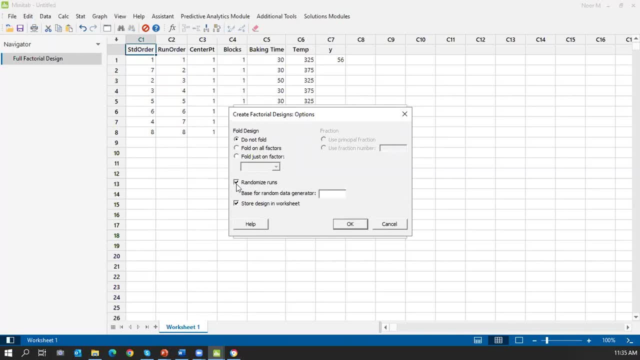 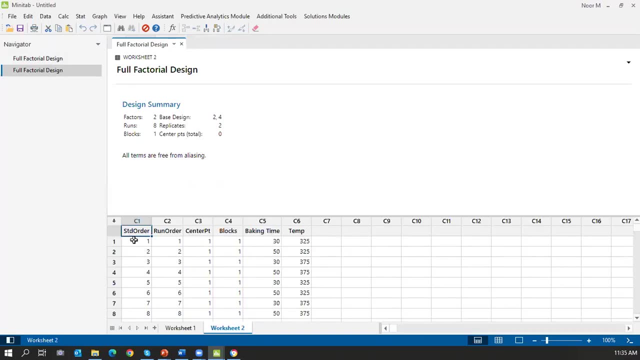 You unclick here If let's say you want the one is randomized, Okay, so you unclick here, Click okay and then click okay, So you will get the same. If let's say you not click and not proceed with the default. 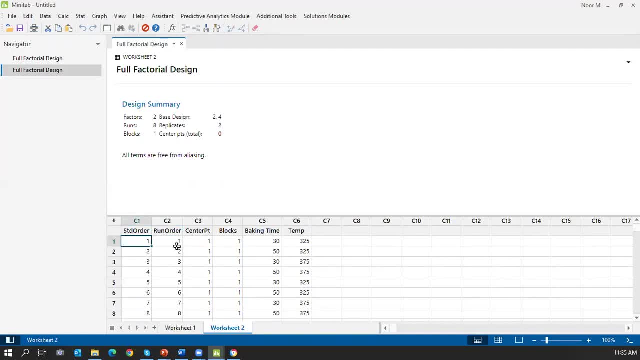 setting. So you will see the run order and the standard order will be the same. Okay, if let's say you choose the randomized, So standard order and the run order is different. Okay, so METEK will randomize for you for this case. 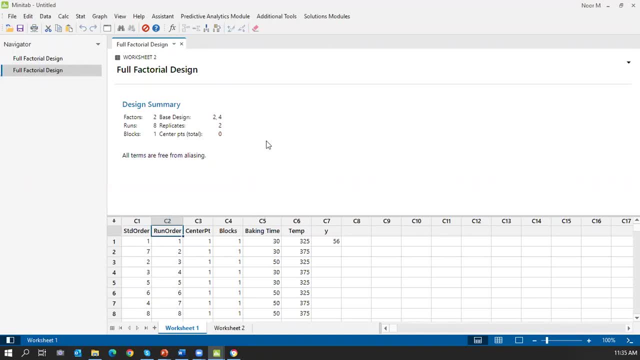 Okay, so this one is how to create the design before you run the analysis, before you run the experiment. Okay, so after you finish all this, okay, you already get the response, So you can proceed with this DOE factory design. You can see now you. 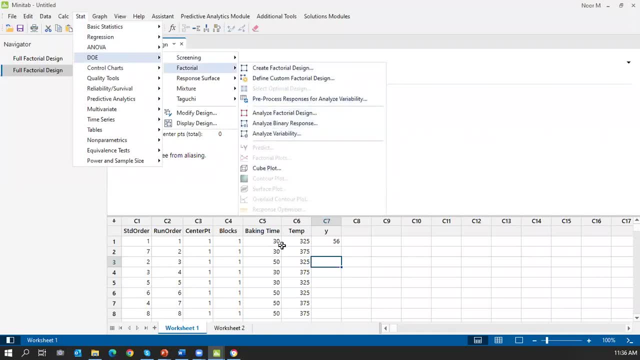 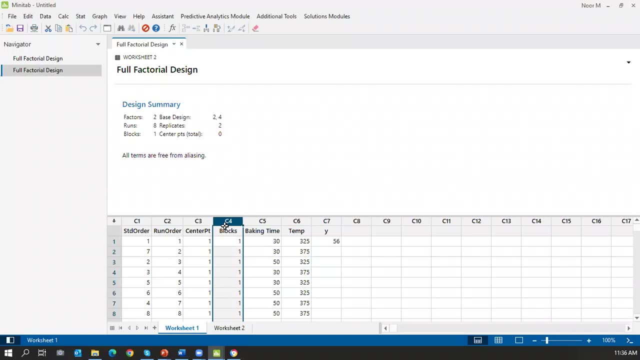 able to click on this one, since METEK already have the design, So must be: start with the define. Okay, create the design. If, let's say, you already create the design in Excel or something that one, and then you put in this mini tab So you are able to see. 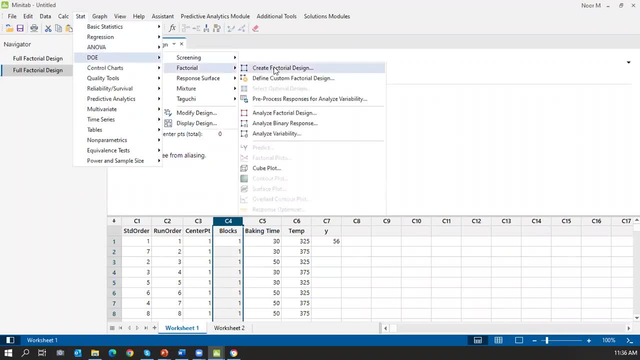 like this one. So go for the DOE. you go for the factorial. define your custom factorial design. If, let's say, you doesn't have any experiment, so you can go for the stack DOE. go for the factorial- create. 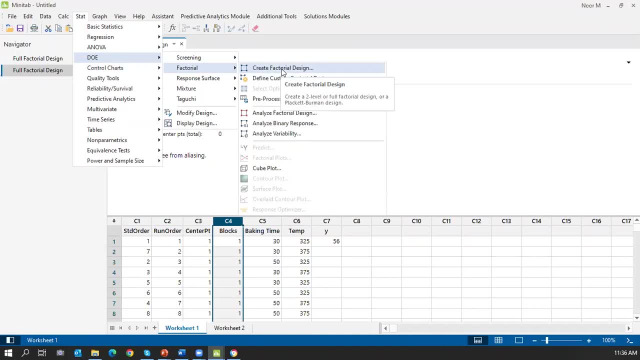 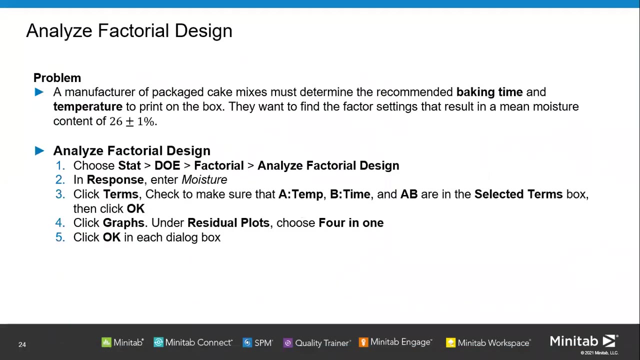 If let's say you already have, you want to do analyze, only so you choose the define custom factorial Same go for the others, design The same step. Okay, so we'll go back to this one. Okay, so we go, we try analyze for this. 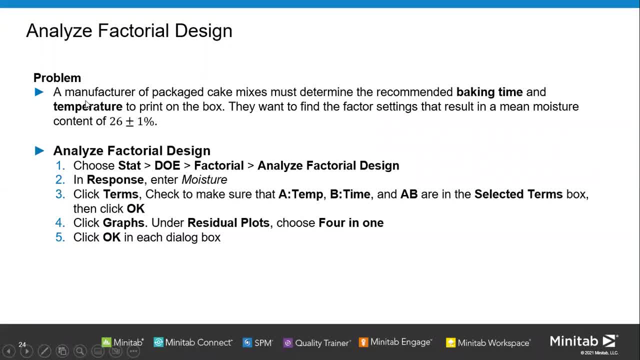 case. Okay. so manufacturer of packet cake mix must determine the recommended baking time and the temperature to the print on the box. They want to find the factor setting. So the result in mean menstrual content about the 26 plus minus 1%. 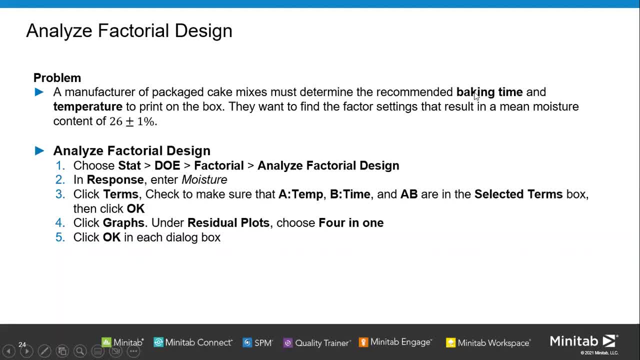 So they will must stick. baking time is 30 or 50, and then the temperature is 3 to 5 or 7 to 5.. Want to that one. So we'll proceed with this case study with the analyze factorial design. Okay, so I will go back. 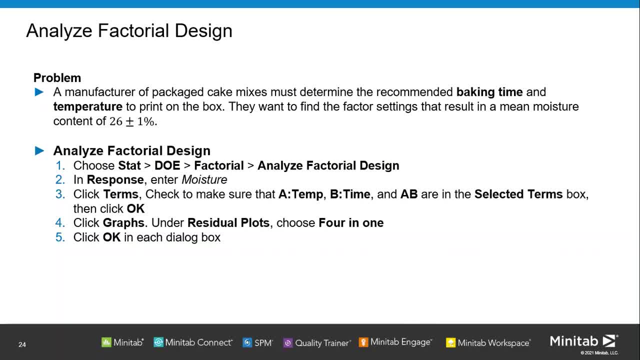 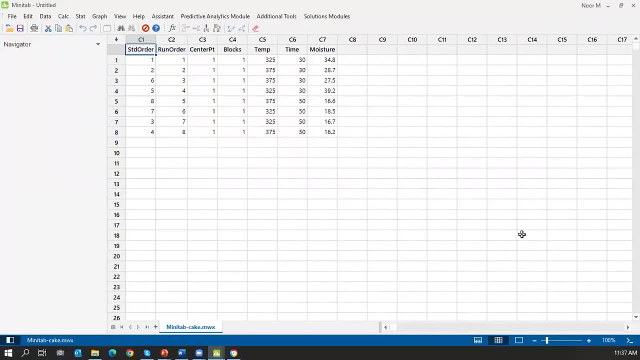 to the mini tab. Okay, you go back to the mini tab. Okay, so I will open this one. So you now your mind, you already run the experiment and then you already have your response. is the moisture For this case? they. 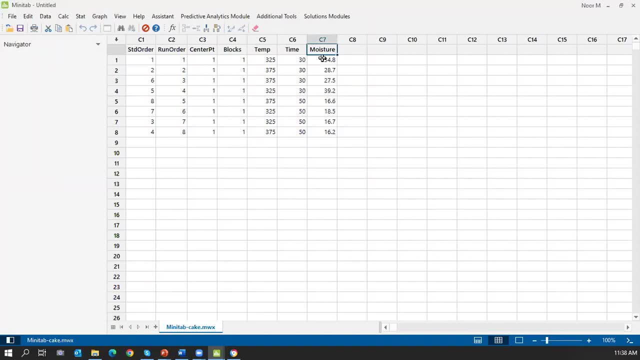 will measure the moisture with the before and after. Okay, after minus before, they will get the moisture of the cake itself. Okay, so how many run They run? 8 run. They work, coming from 2 replication. So how to proceed with the 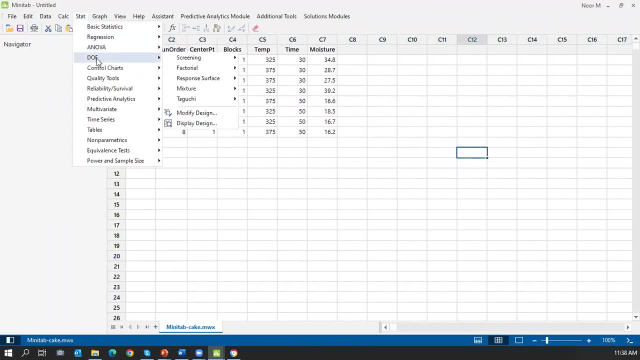 analysis. Go back to the stat. go for the DOE, go for the factorial design. You choose factorial design: Okay. but if let's say your Y is start measurement, you can choose the DOE, factorial design. you choose binary response: Okay. 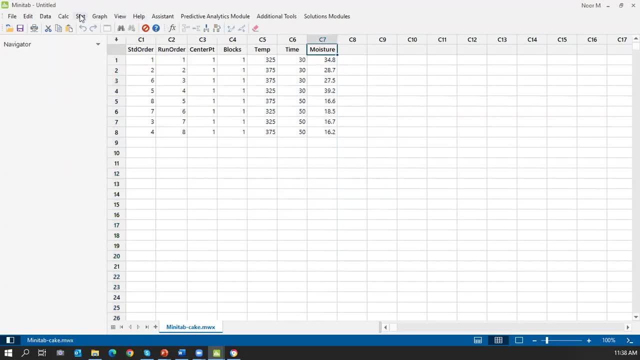 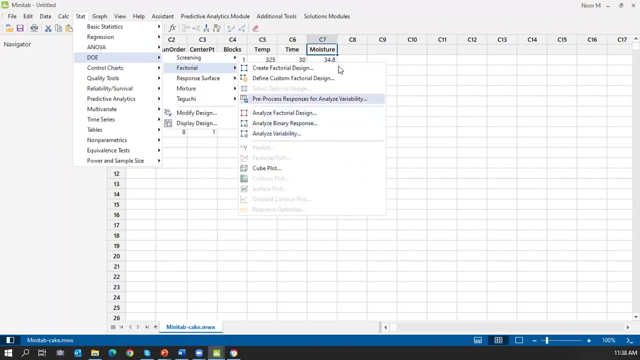 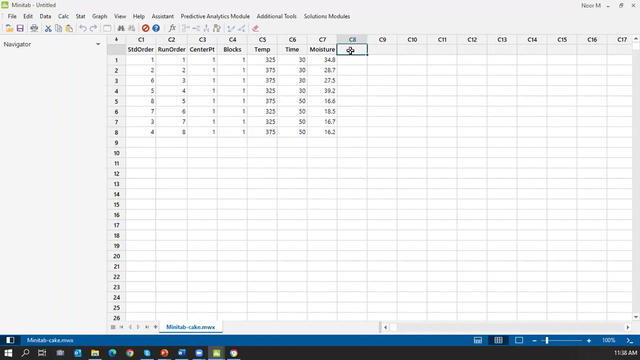 so if, let's say, your Y is 1 and 2, you can go for the DOE factorial design. you choose variability. Maybe you not only measure on the moisture, maybe you measure on what type of that one is a weight, maybe something like that one and so. 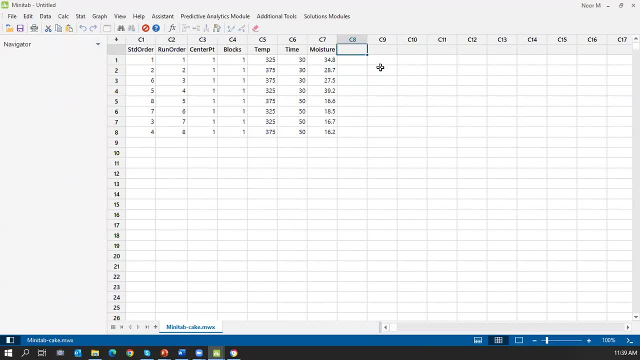 on. So they will be. analyze variability. So we have a different response measurement. you look on this one For this case. we try with this DOE factorial design. we choose the factorial design. For this case, our response is the moisture. 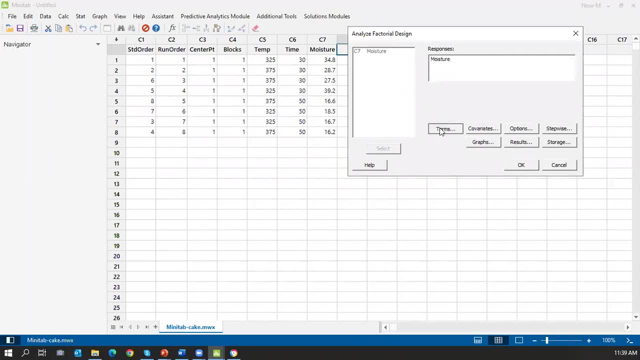 So you go for the moisture And then the terms. here you will look on the what For this case, we will look on the temperature, we look on the time and then we look on also on interaction. So that's why we do. 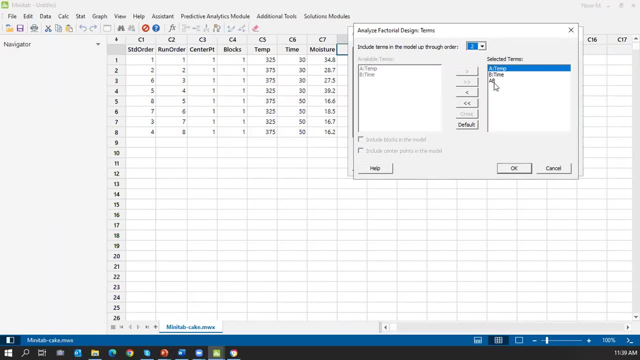 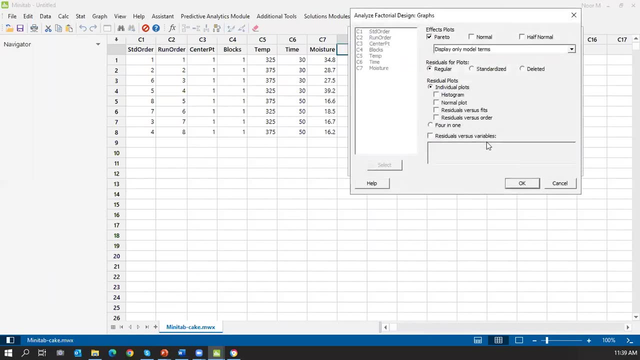 the DOE, We choose the factorial design. for factorial design We want to see on the interaction, Click okay. and then of course this one is a statistical, So statistical tools, so you must be an assumption on that, So you click on the. 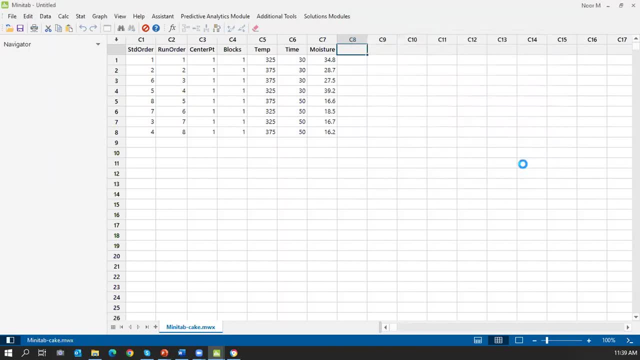 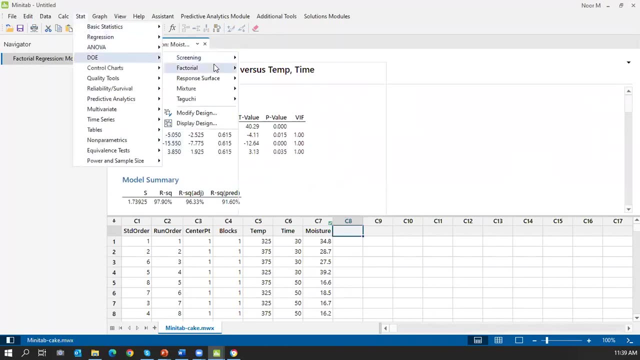 factorial For each one, click okay. and then you click okay. Now you will get the result on this one. I will do. go to start, go to DOE, go to factorial. You can see on the analyze: factorial. So you must decide your response. 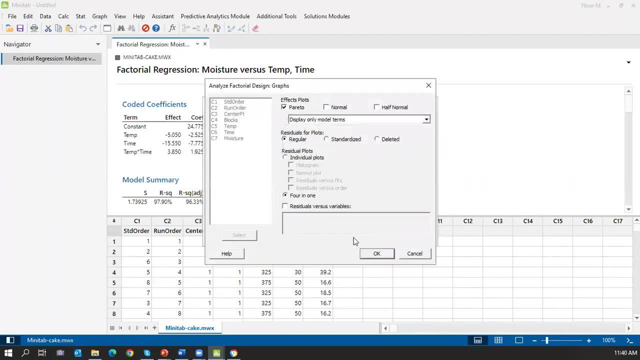 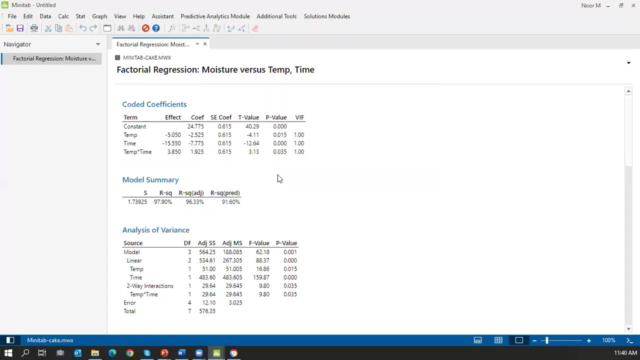 your terms here and then you click your graph and then you click okay, and then you click okay, So you will get the result for this case. On this one, of course, we want to see on the what, which one is a backing time or? 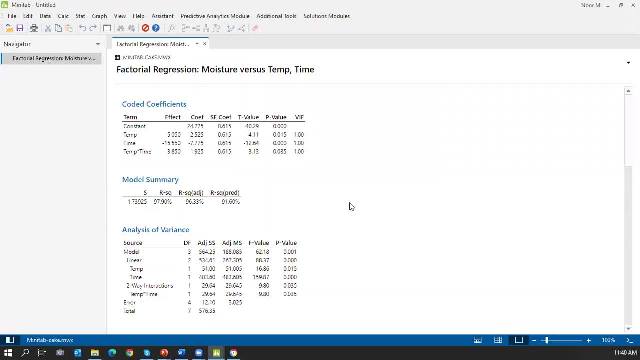 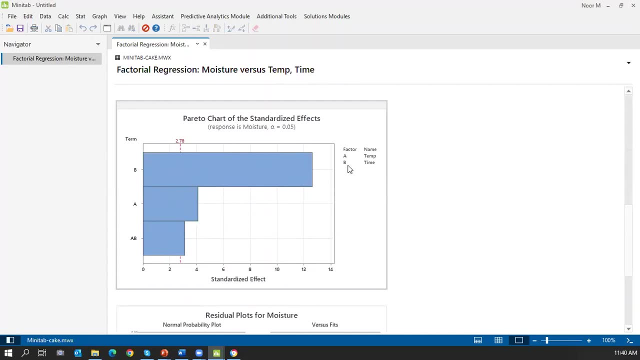 temperature, It will most impact to the moisture itself. So maybe you can go for the Pareto chart. So, based on this Pareto chart, all the factor and then include all, include the interaction it will be significant to the moisture itself. Okay, 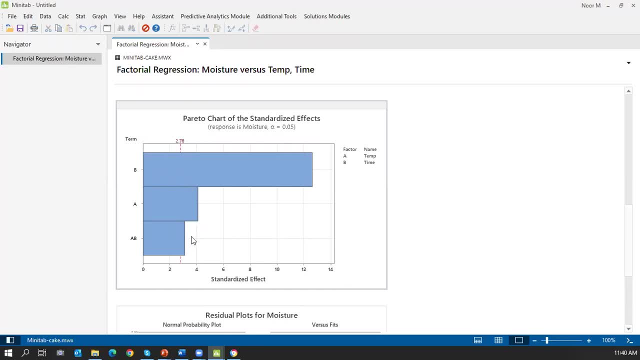 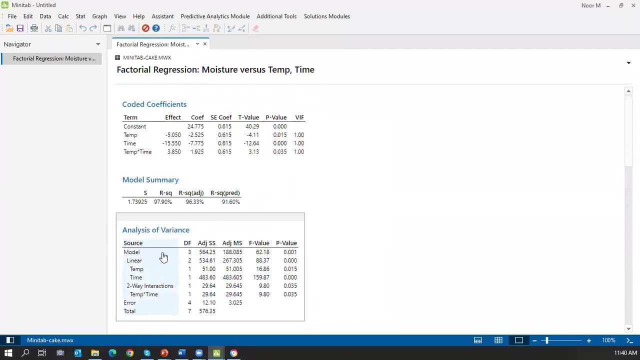 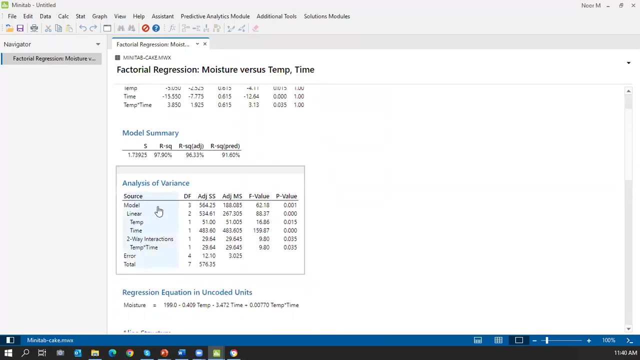 So from here, okay, both of the term is a significant interaction for significant. So that's why you need to look on the analyze, Okay, And over here, So maybe this one is a visualize. Okay, You will confirm it with this. 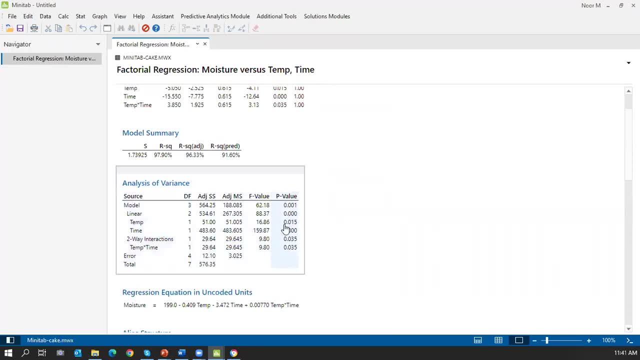 and over. So, based on this and over, you look on the p-value So you can see the p-value is less than 0.05.. So we need to say that temperature is a significant time, also significant Interaction between them. 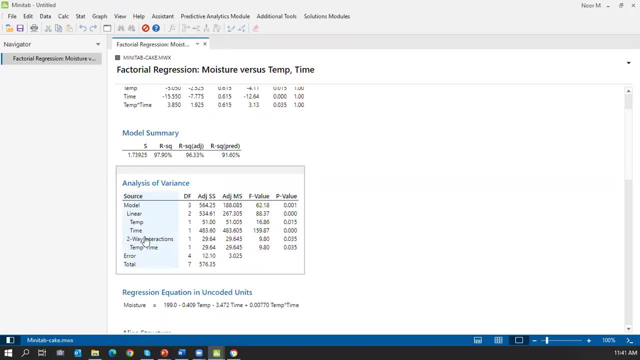 also significant. But you remember that In the temperature you have a two level, which is a 30 minutes and 50 minutes, And then for the time- sorry for the time- you have to 30 and 50. And then the temperature you have. 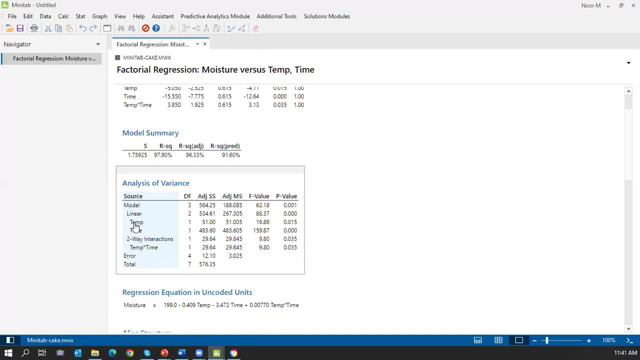 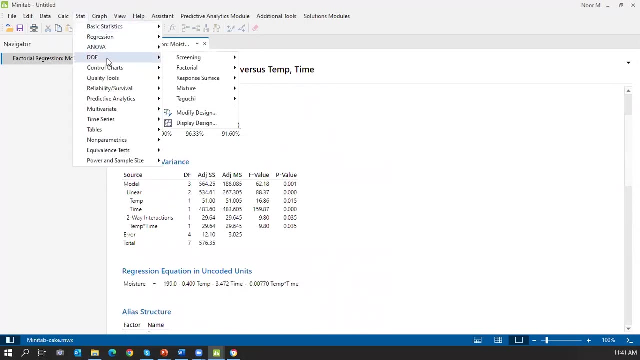 a 325 Fahrenheit and a 375 Fahrenheit. So which one is most important? level for temperature, most important level for the time. So we go further with this, Okay. Next one: go back to the DOE, go back to factorial design. 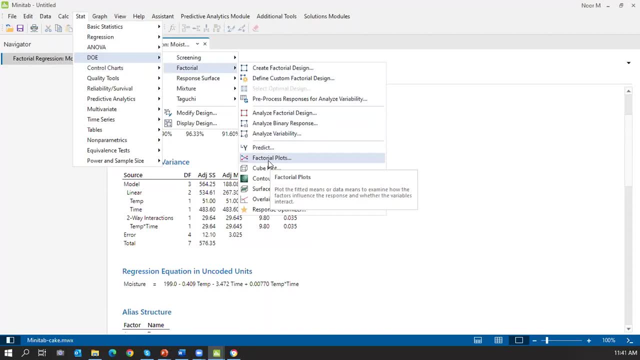 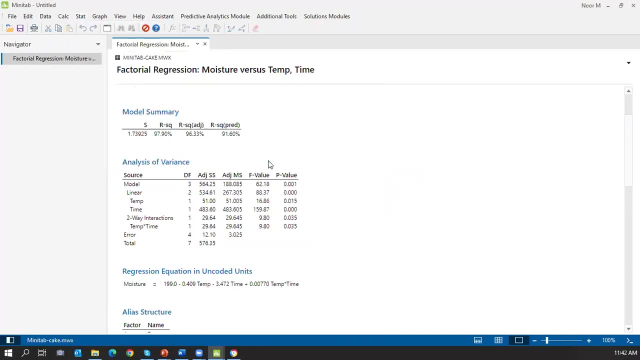 So you can go for the factorial plot. Okay, So now time. temperature interaction is important. So you go to the factorial plot And then you can see that this one is this time Okay, And then temperature, and then you click okay, So you will. 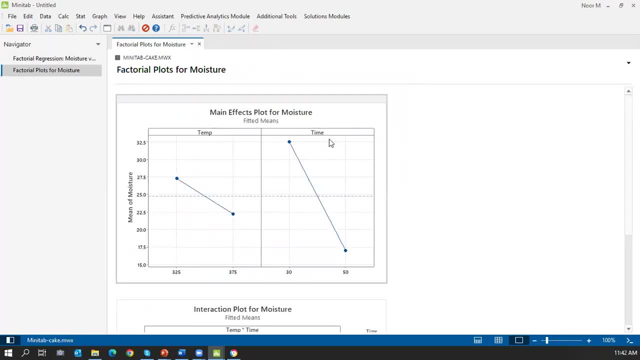 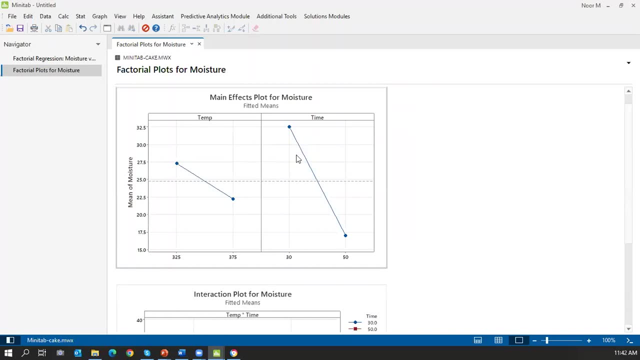 get the most impact, most effect of the temperature and most effect for the time. So based on this, okay, you can see that the highest value of the moisture is at the temperature, at the lower temperature. Okay, The most high. 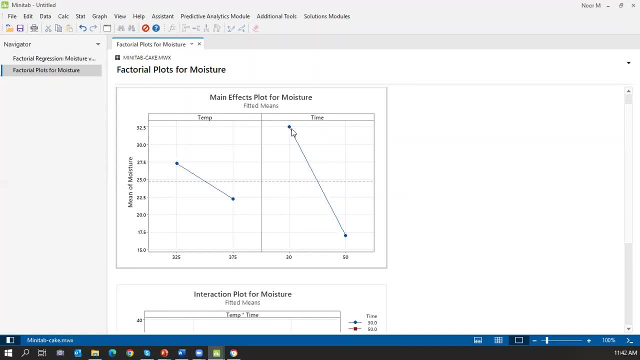 the most higher of the moisture is the low level time. Okay, Less time will highest the moisture, So less temperature will make it higher. So we have the main plot here to see, to give it to you which one, which level for each. 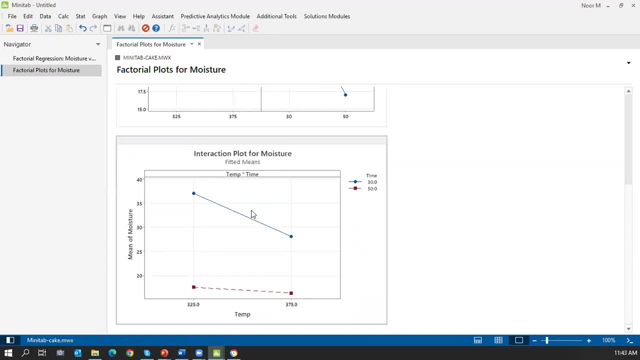 time, And then you can go for the interaction here also. So, based on this one, they will have an interaction between them. Okay, Between the temperature and the time. Okay, So after that we can go for another way. Maybe you can. 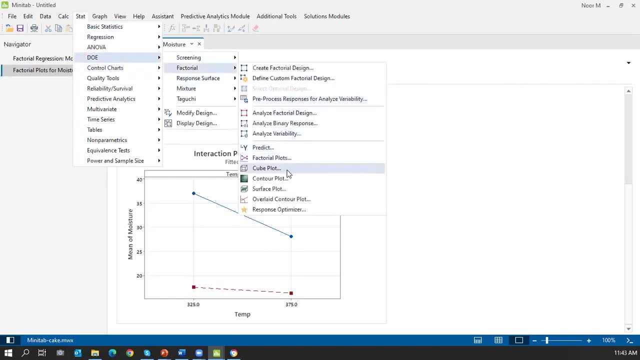 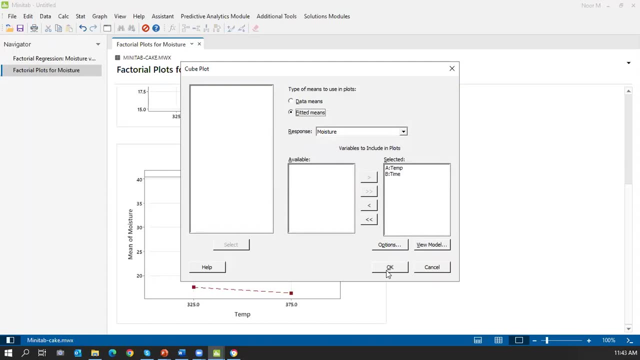 go for the design experiment tutorial. maybe you can go for the cube plot. Okay, Cube plot for this case. Maybe you have fitted one and then you click okay, So you will show or visualize your finding with the cube plot here. 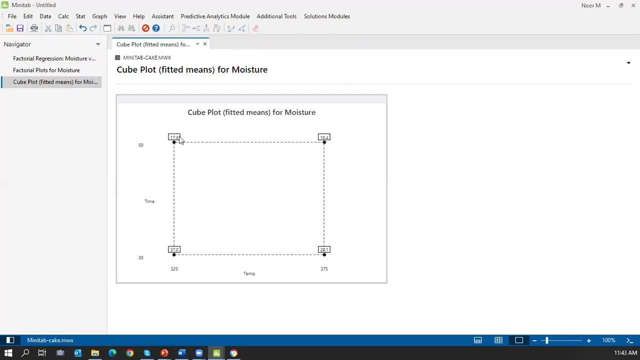 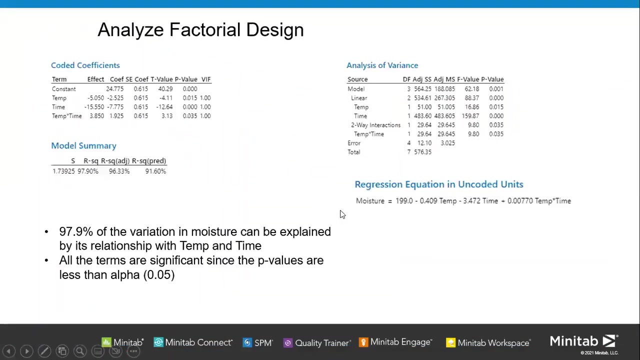 So with this 50 time minutes, this one is the moisture, This one is the temperature: 325, 375.. So all this one, I will go to back To this. Okay, Already done it. Yes, this one. 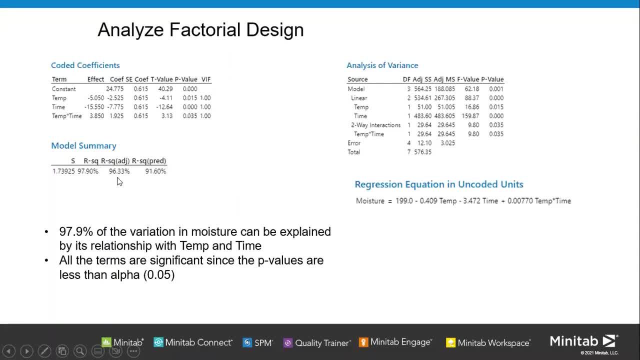 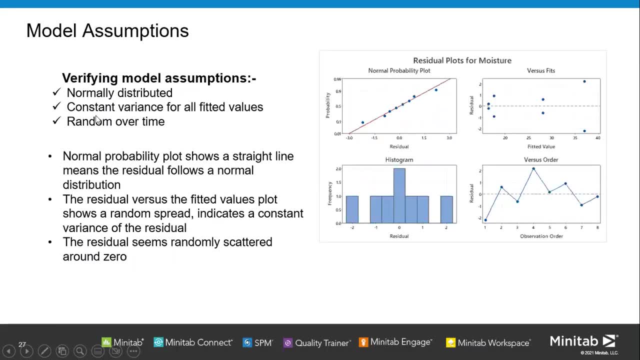 And then we look on the model summary. Okay, So you are out squared here, So it's a good one. Okay, More than 70.. And then you verify the model itself. Okay, So, since this one is the statistical tool. 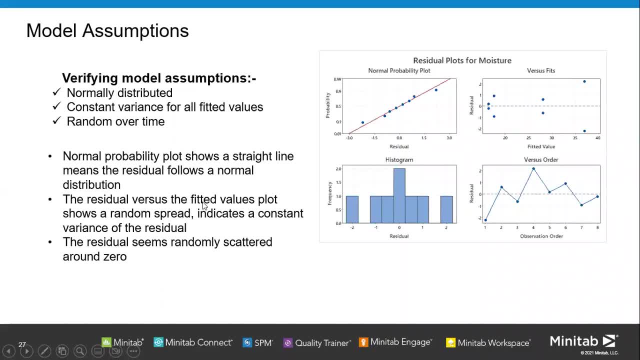 so you cannot avoid this thing. Okay, To rely on or to validate your result. So must be: look on the normal distribute, must be look on the costum variation and then the random over. So all this one is a good one, Okay. 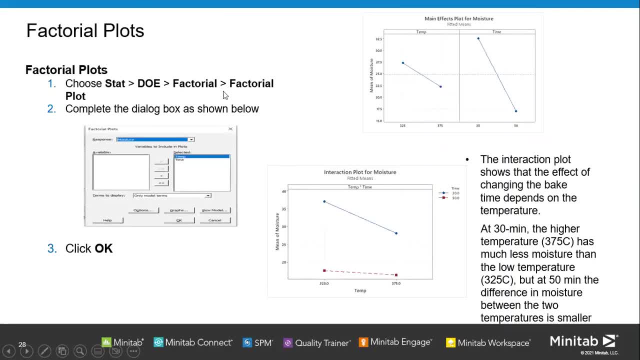 And then you can proceed with the. just now I will show the interaction plot. Okay, So the interaction plot show that the effect of changing the big time depends on the temperature. So if let's say here you can see that Okay. 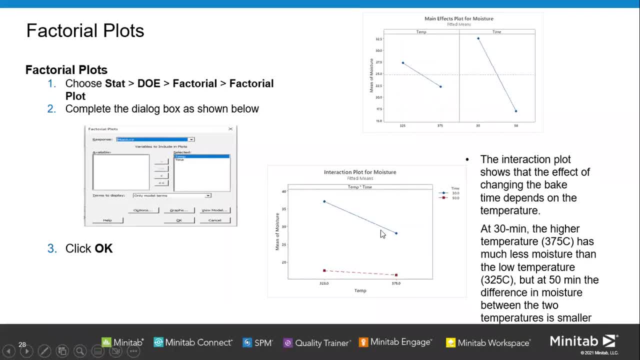 It's something like differences. Okay, So when temperature is high, Okay, And your time is a low, Okay, So will lower, better than temperature. low, Okay, The height, the the time is higher, Okay, So at the 30 minutes, the higher. 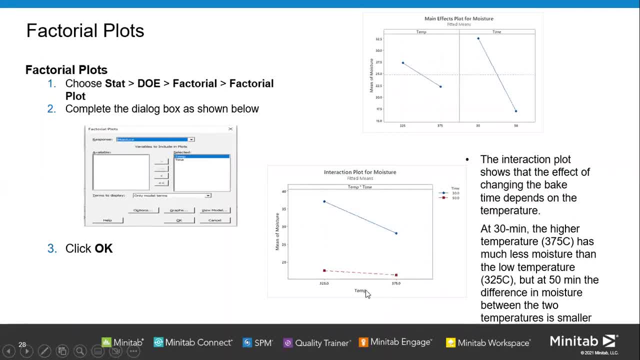 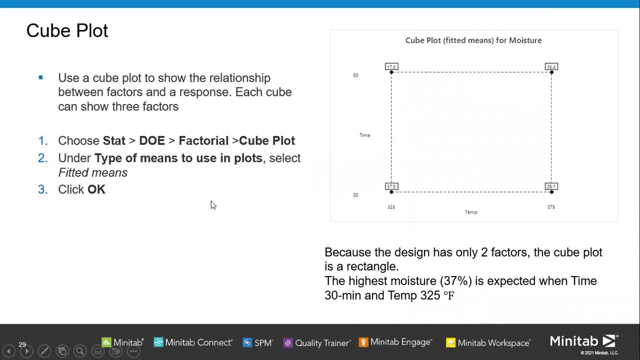 temperature has the much less measure than the lowest temperature, But at the 15 minutes the differences in between them is smaller than one. So this one, Okay, And then after that maybe you can go for the cube plot. Just now I will show how to get it. 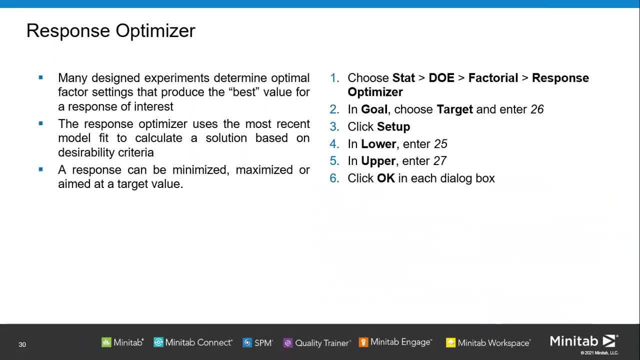 This one, And then, of course, this one, the last, the last aim of this project. Maybe you want to. how about the many design experiment determine the optimal factor setting that produce the best value for a response of interest For this case? 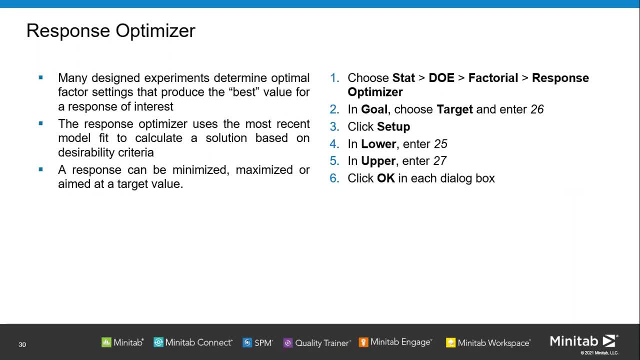 of course we want to know about the moisture. Okay, The response itself. use the most recent model fit to calculate a solution based on the disability criteria. A response can be minimized, maximized or aim at a target. So just want to highlight. 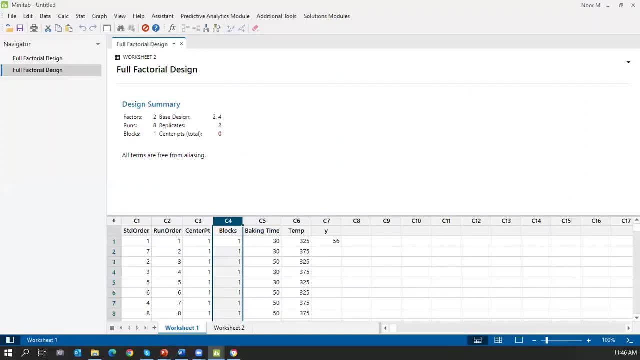 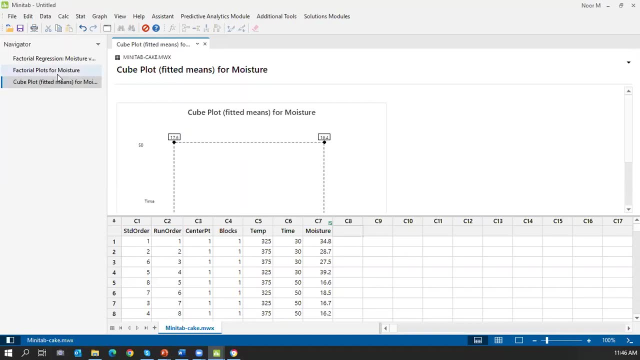 since this case study, this case study already good, is a good model, Okay. So if let's say, you pick up, go back to this one, It's good model. Okay, It's good model with this R squared. And then the assumption, also the fulfill. 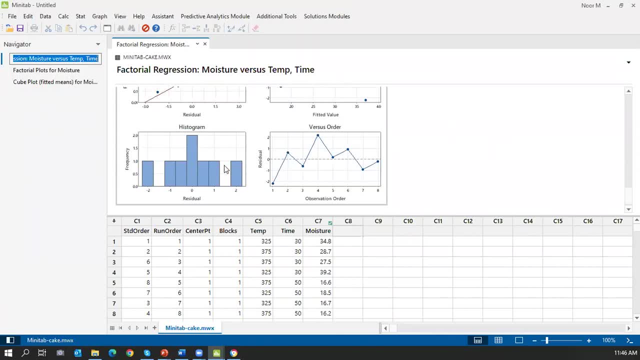 So you no need to refit the model. If, let's say your, your, your experimental is not so good, Maybe you reduce the number of factor, reduce of number of interaction, So you might be refit the model back. 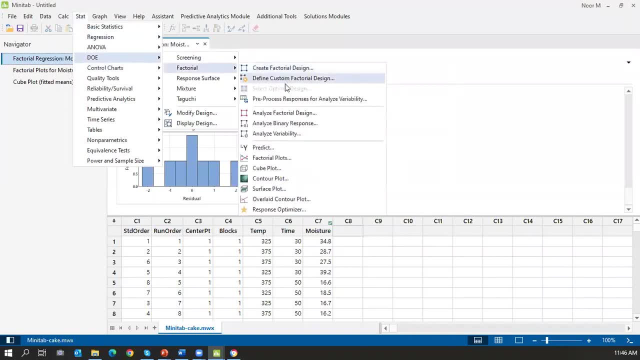 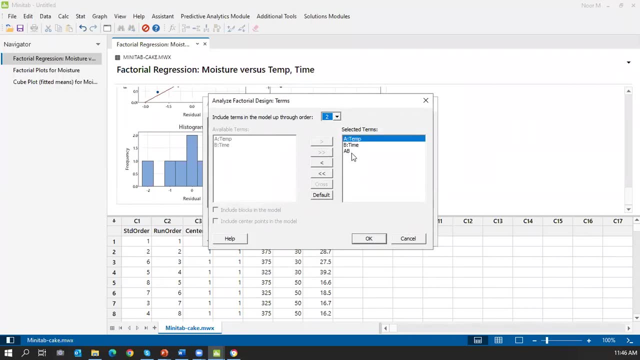 So go back to the DOE, go back to the factorial, go back to the factor analysis. So lose on this one. So make sure only significant factor be available on this selected terms. Okay, So that one, since this case study is only two. 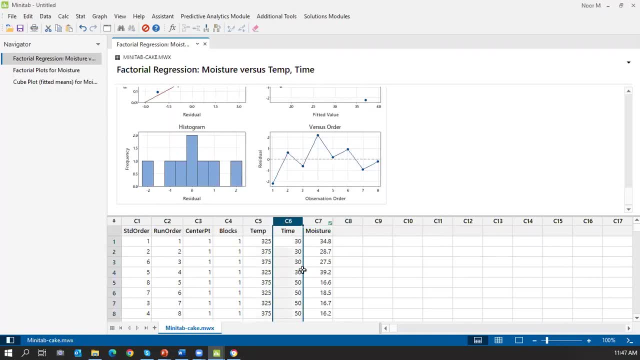 okay, it's only two factor, So maybe it's not so complicated. Okay, Maybe after this you run your your own project like five, five factorial, So it's something like it's a complicated one. Okay, Not only two duplicate. 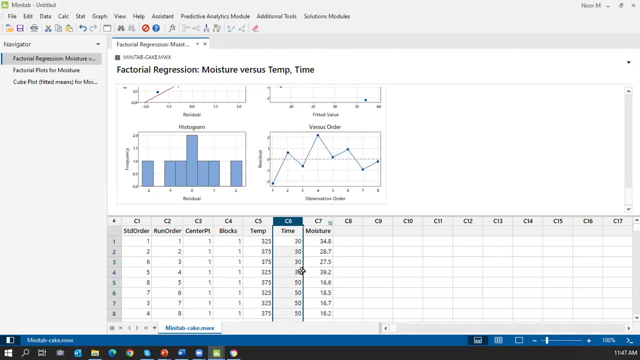 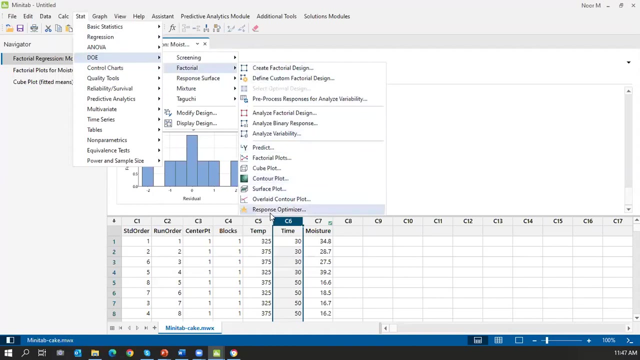 maybe more than two, more than three, duplication, So it's more complicated. Maybe you cannot be a straight way like this one, So you need to refit the model before you go back to this. DOE, optimize them. Okay, So response optimizer, this one. 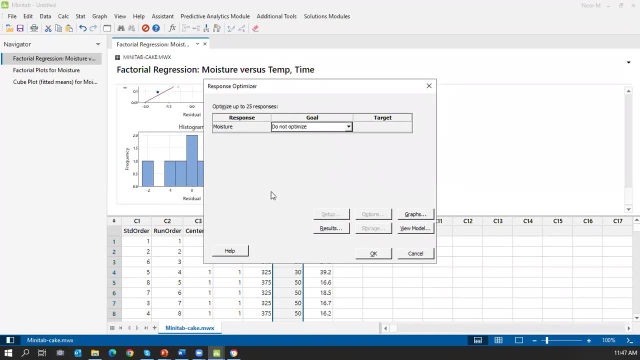 Okay. So before that, one Minitech will re-trigger the last, the last part of the model. Okay, You refit, refit, refit, and then you will consider on the response optimizer Once you create the optimal optimizer. 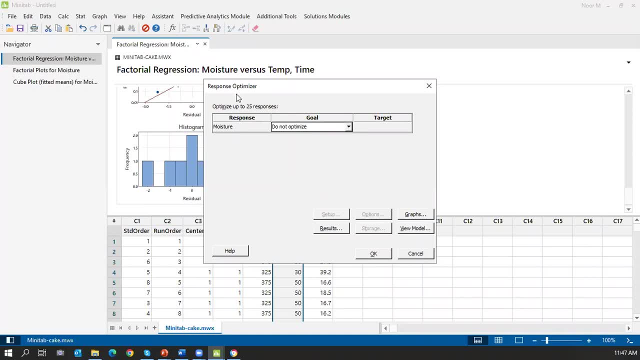 Minitech will trigger the last part of this, Okay, In the response optimizer. So you will be care about this one, Be aware about this. So you refit, refit the model, you change the model, you change the model and then 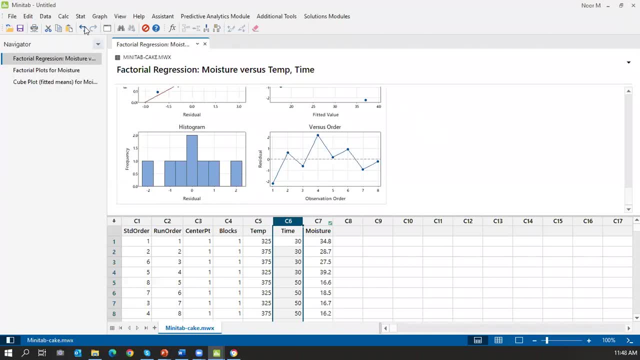 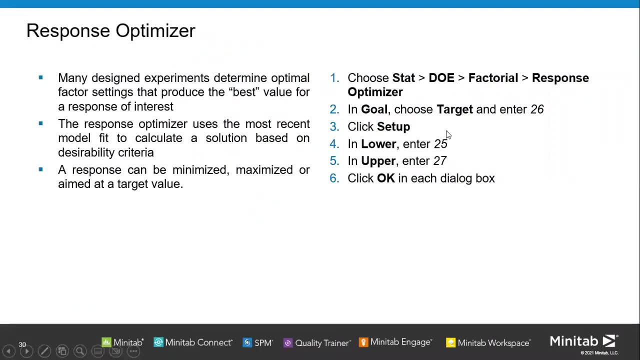 you make it clear what is the best model And then after that you can go for the response optimizer, This one, Okay. So for this case we try with the target itself. We have a target. your, maybe your- spec meet the target. 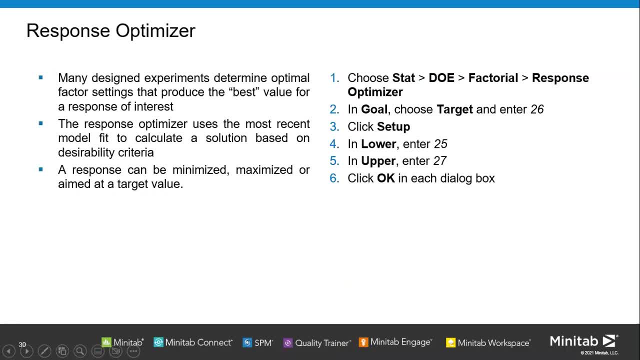 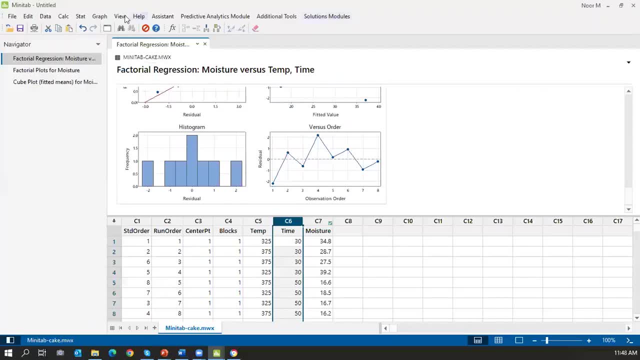 and then the lowest, the enter and this one. So I go to the Minitech. Okay, Go back to the Minitech. Okay, So go for the stack, go for DOE respond, and then I will choose the. 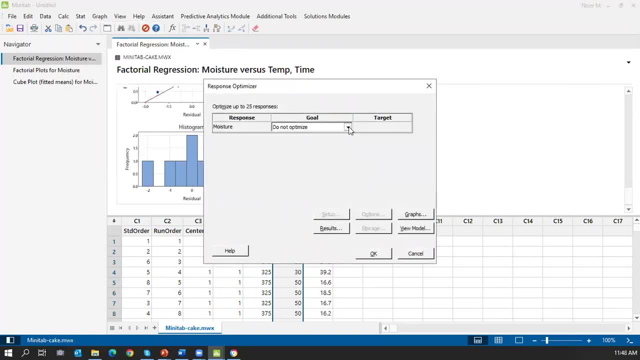 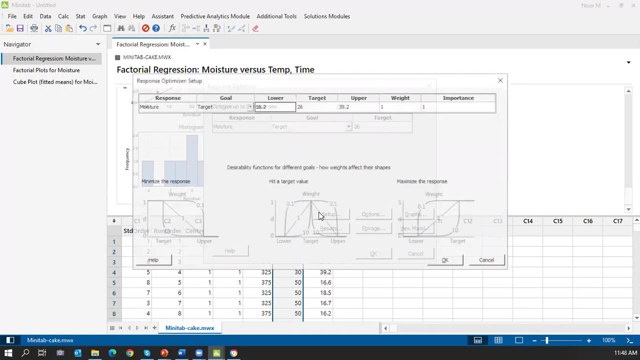 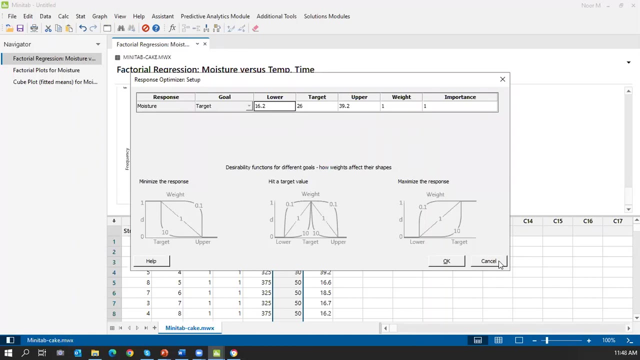 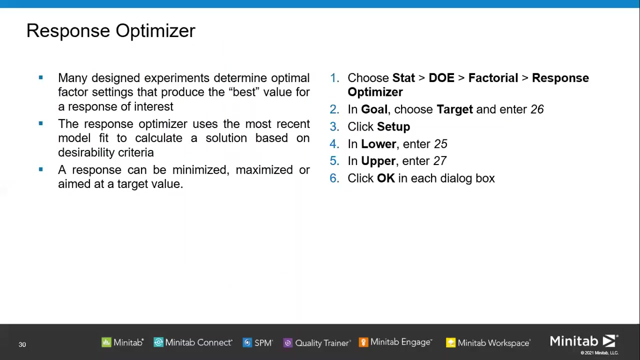 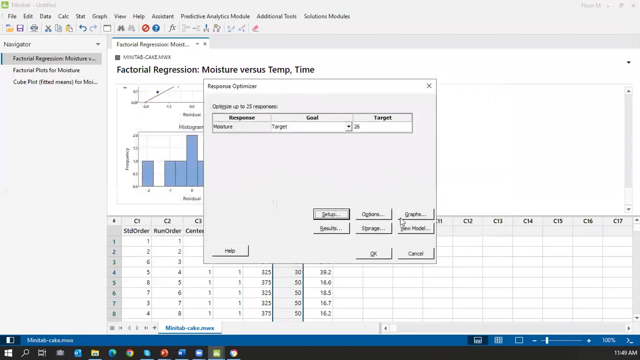 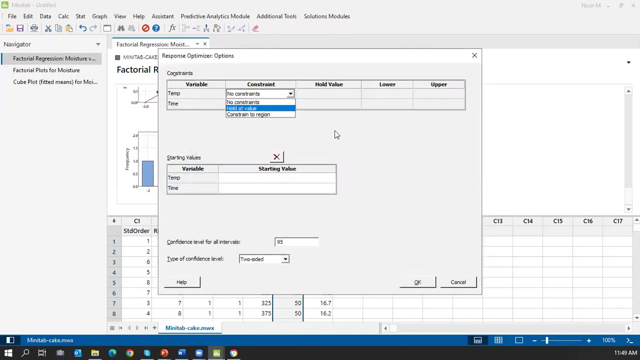 response optimizer For this case, we won't have a target. Okay, our target is 26.. just set up here, okay, so it's the lowest, the slowest, sorry, okay. and then your option here: okay, your temperature, your constraint here, hold at a light or something, that one. i just proceed with this one on me and then maybe 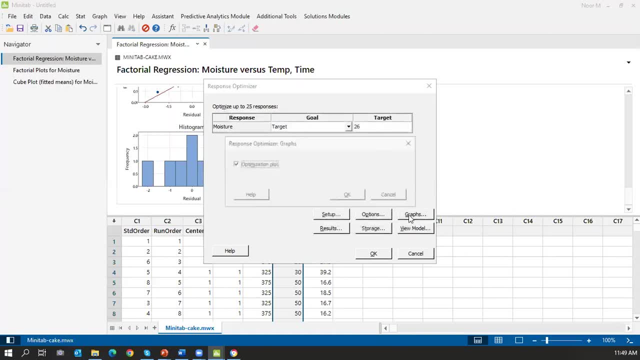 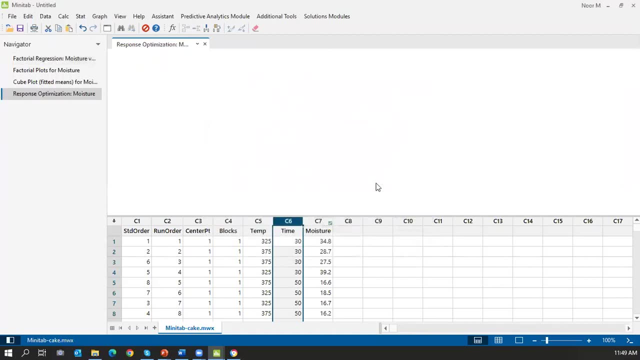 you will go for the result, okay, and then you go for the graph itself. then you click: okay, okay. so your, your objective is the on the target, okay, on the target with this target, okay. and then here is your feed, okay, feed. and then this one is your response, this is setting here, and then you 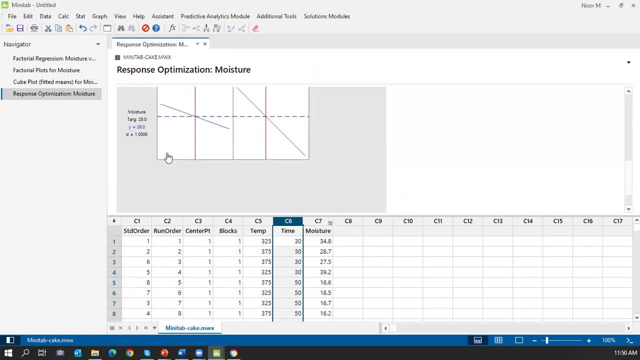 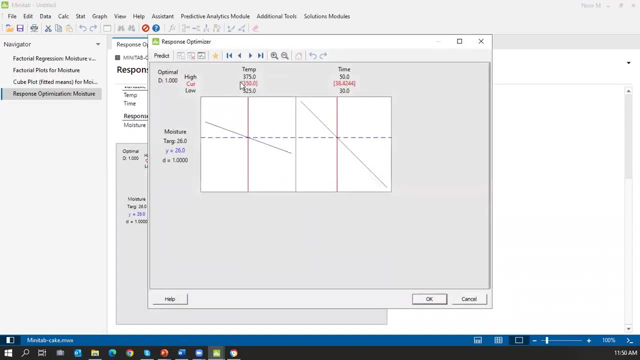 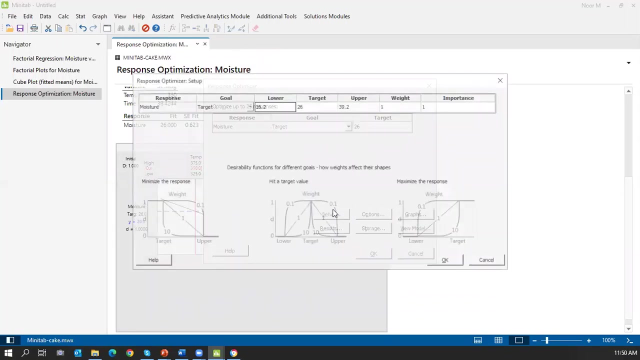 will get the optimize this one. so actually you can uh okay. okay, you can uh set it up for this case: okay, the highest or something, that one, so this lowest. okay, you can manipulate for this case. okay, double click and then you click on this one. okay, so i will go back to this dialog box. your target maybe you'll set up here: okay, the lowest. 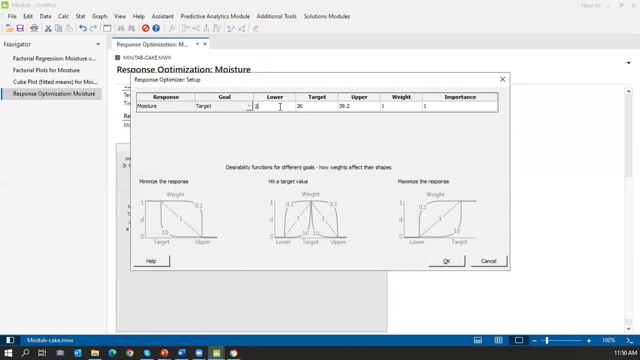 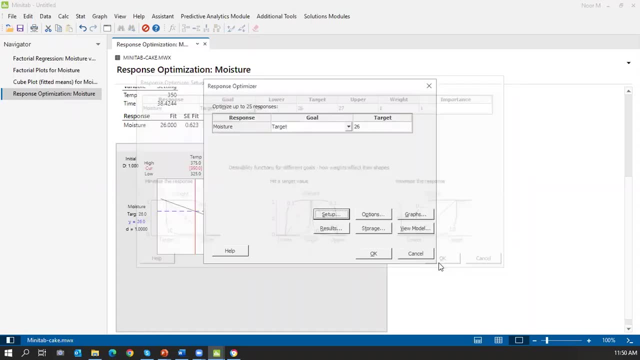 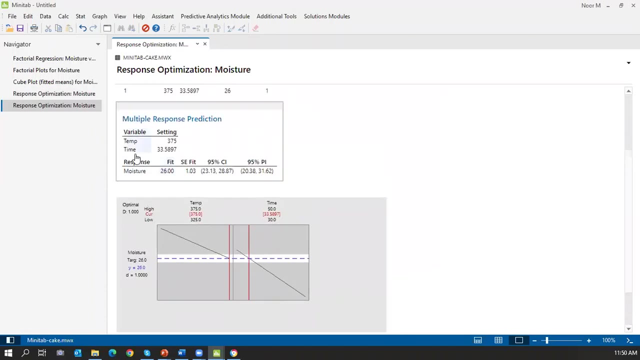 maybe here is 25, okay, the upper here maybe it's 20.. seven, and then you click okay. so you click okay, so you will get this setting. okay, so you will get this one, the fit between this one, this setting. okay, the best thing if let's say: 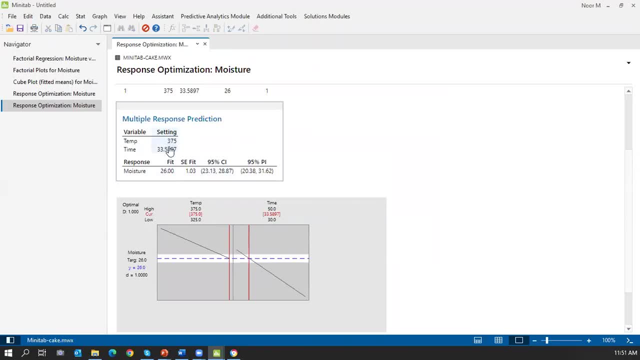 you want to. the target the voice is that your temperature is 375 and your time is between 30.5 eight nine seven. so this one, it will be print on the box. okay, so this one is how you want to use the mini uh doe to solve your problem. the first, we create the design. after wiki design, we run the 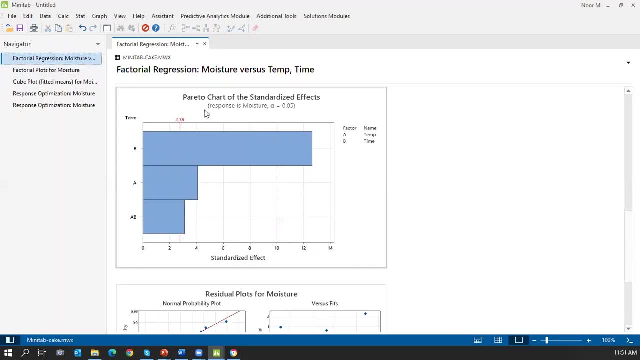 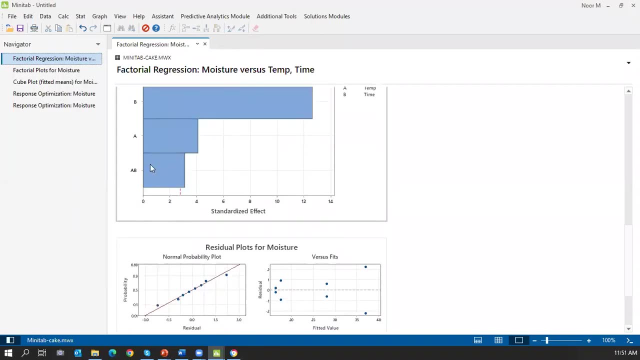 analysis. after, during dry analysis, you will get with what factor is a significant and what level is the most important. after that you will try. then you can go and get right. theWhen do you use CLI generate process for the dose of Receiving Test? then we will use what is the dose and what is the value for body temperature? I think with your clicking on that, înot how to print on the box. okay, so this is how you want to use the still mini DOE to solve your problem. the first we create the design. after we can design, we run the analysis. after, during Hepat, theeевой will get what factor is a significant and what labor is most important. after that you will try to use 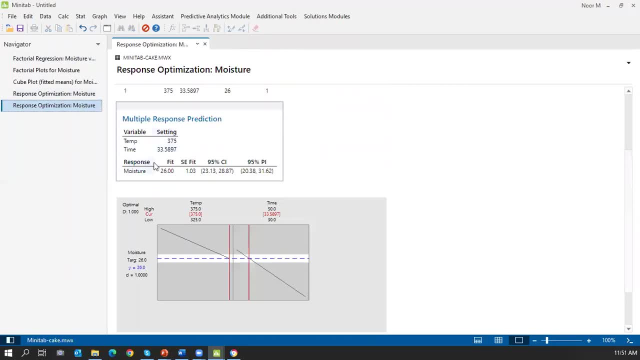 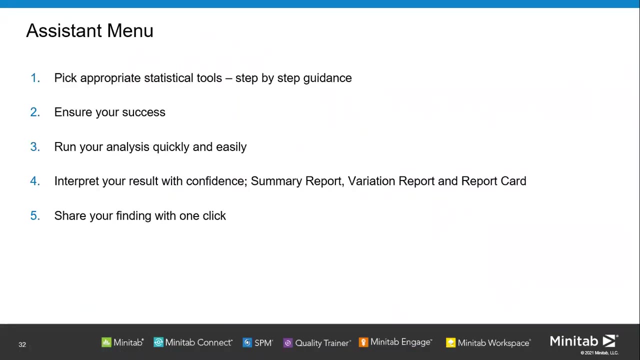 you will try to optimize your setting and then you will get the setting for each of the variables itself. So we have another way to get the DOE in the MINITAB so we can use the assistant. But the assistant- we have a limitation on that. 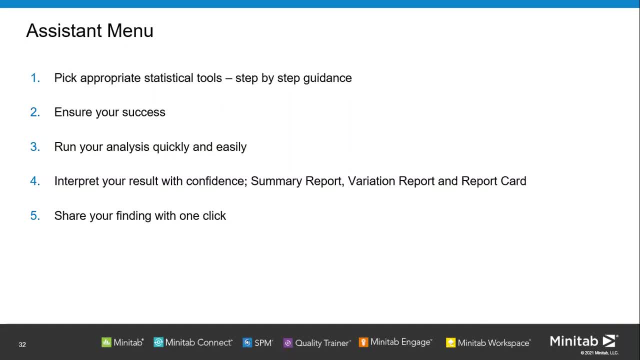 If, let's say, you have a more than five factor, so you're not able to use the DOE in assistant, So you need to back to the DOE in the step menu. So that's why I always suggest you try with the step menu first. 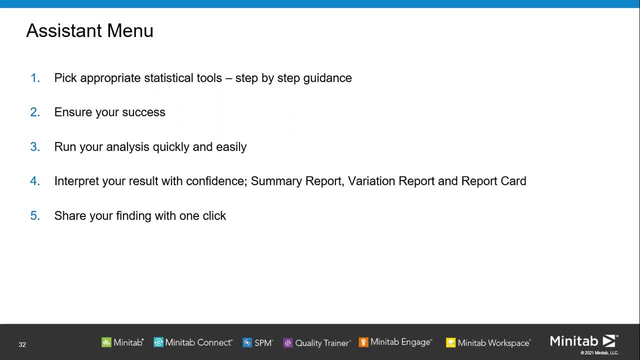 And then if let's say, just only reconfirm, just only to study so you might be, use the assistant menu, So it will work like the same, So it will work like the same, So it will work like the same. 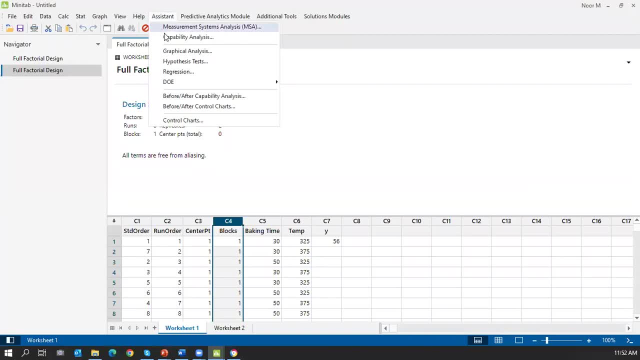 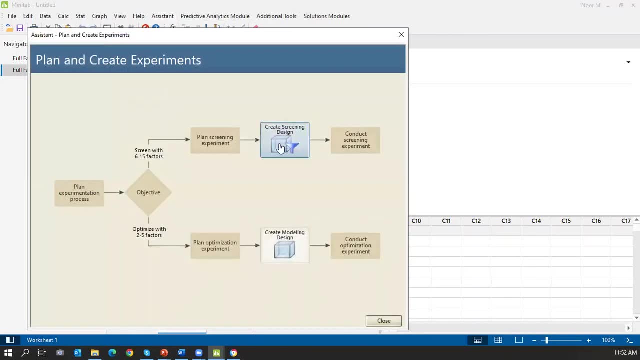 So you can go for the assistant, Okay, you can go for the assistant, You can see the DOE and then you can see that discipline and create. So whatever we do, we need to create the design first, as a previous one in the step menu. 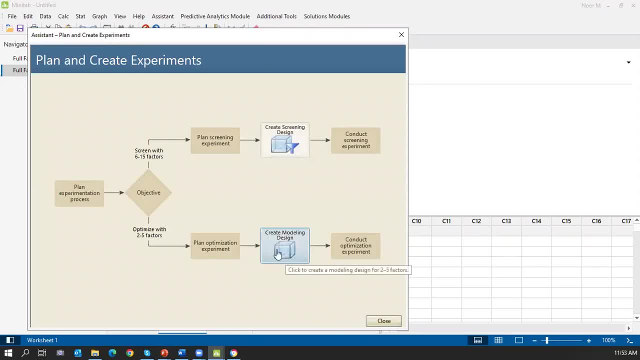 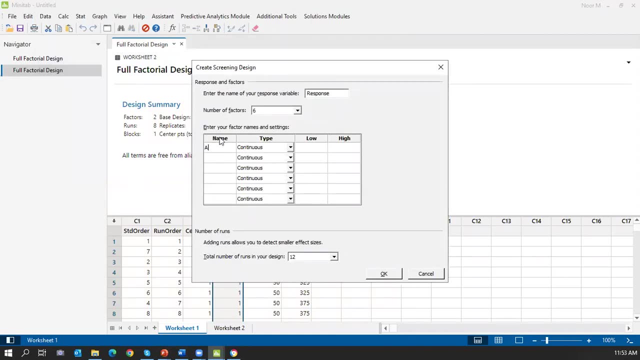 So you need to create all the design first And then after you create okay, for example here, after you create okay. So for first case is A okay. This one is a B name for the factor six factor, because here we use the six factor C. 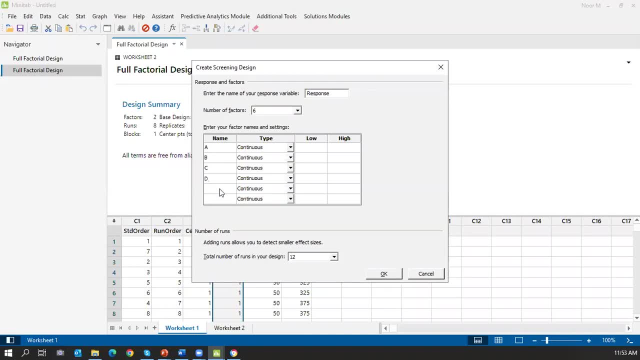 Okay, and then here may be one. sorry, here may be negative one, Okay, negative one. here is a one negative one, And the other is C negative one. Okay, another one, yeah, two. it is negative one, negative one. 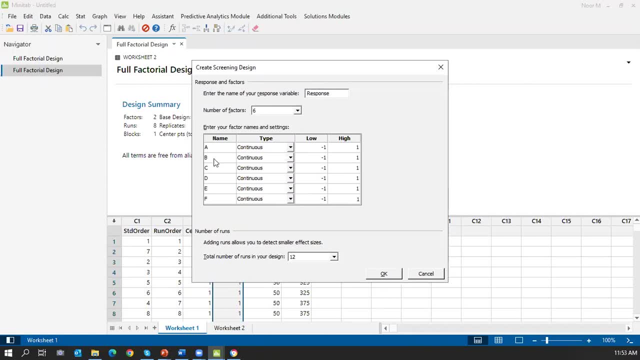 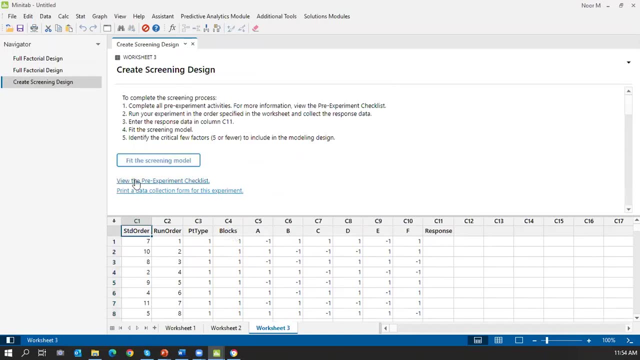 You up Okay, so you respond. so how many run is a 12 run? then you click okay, Okay, so now you using the screening model and then your respond. So after you have the first run, here is a A. 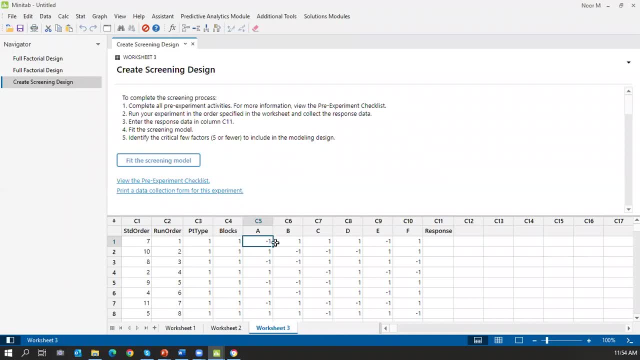 A. Factor A is a negative 1, factor B is a: 1, C1, D1, E negative 1, F1.. So this combination, what measurement you will get? So, for example, it is 77, and so on. 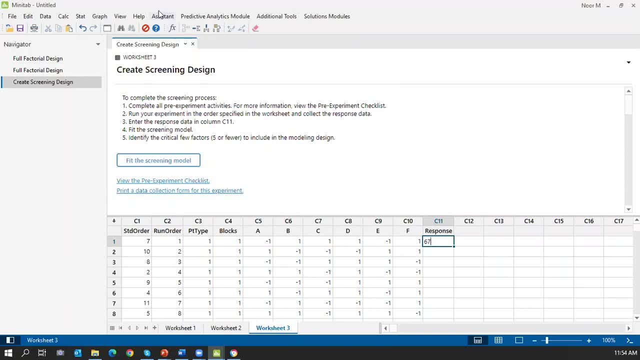 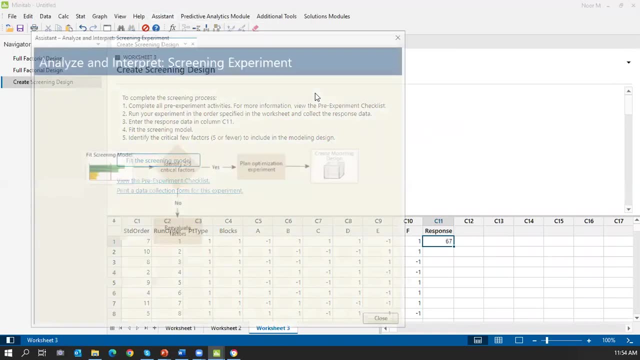 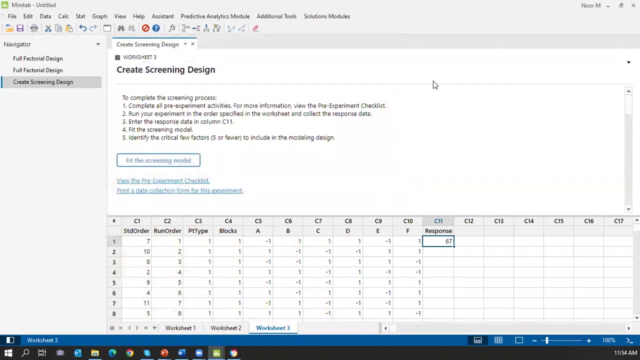 So after finish all this, you come back to the assistant and then you can go for the DOE. You can see the analyze and interpret. Okay, you can see the analyze and interpret for this case. Okay, for this example. I have the. 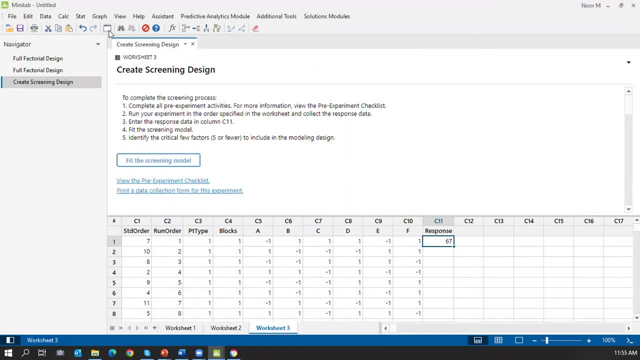 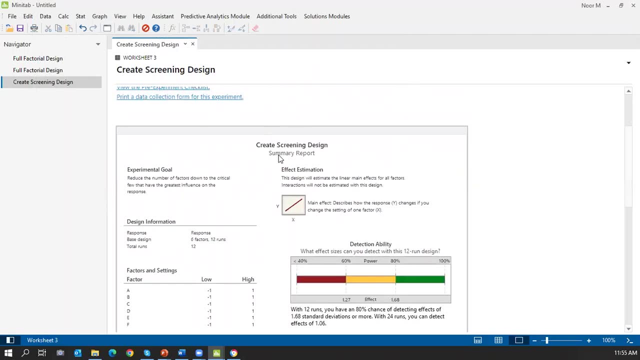 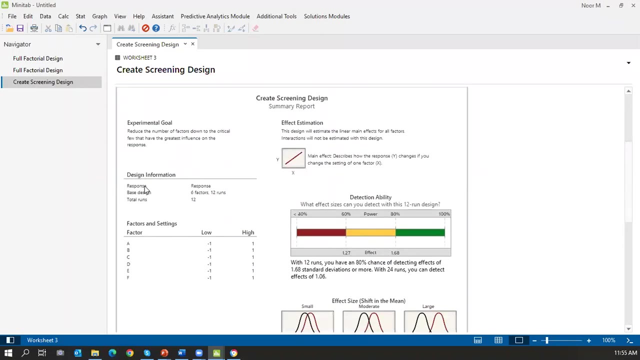 screening. So go back to this one. Okay, for the create itself. they will the same. Will we have a summary report? You will have a report card. So in the summary report they will use the what the design information. 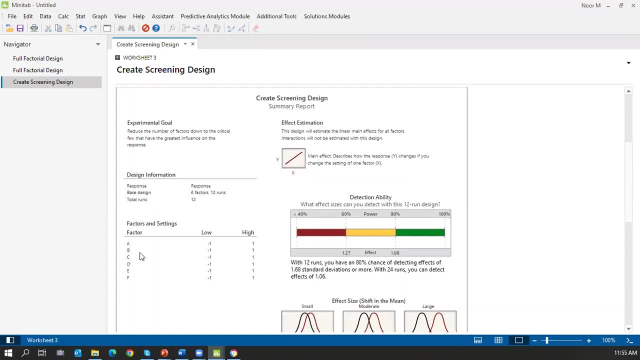 how many factor you have, how many run you have, and then the setting factor here, And then this one is the effective. okay, effectiveness of your number of run, Okay, and then here is the moderate, small, large. They will give it you. 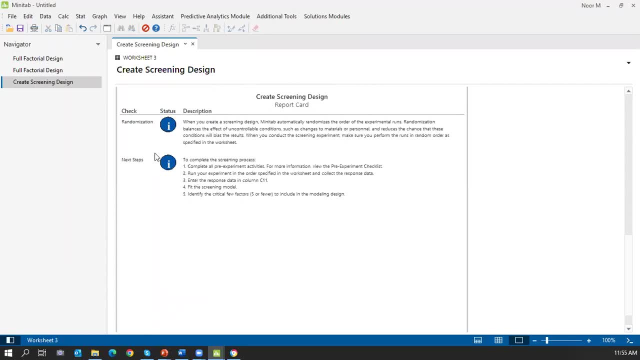 This is randomized size And then the next step. they will show you the next step. What is the next step? So you need to run, complete all the three experiment activity, Run your experiment and then after that you can go for the analyze here. 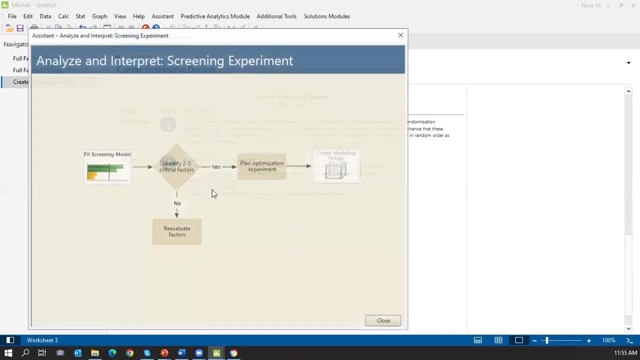 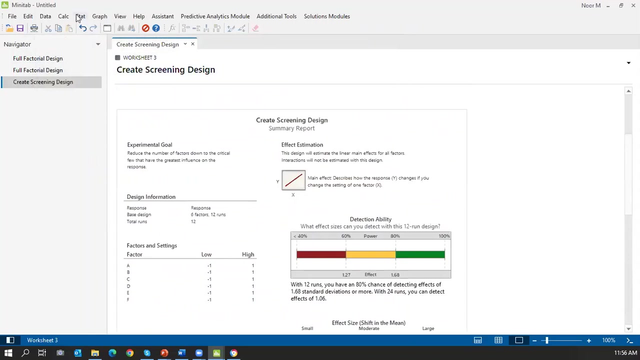 Okay, back to the DOE: analyze and interpret once you're already done for this case. Okay so, maybe it's not satisfied, You can go re-evaluate for this factor. Okay so, not only understand menu, but you will use the DOE using the assistant. 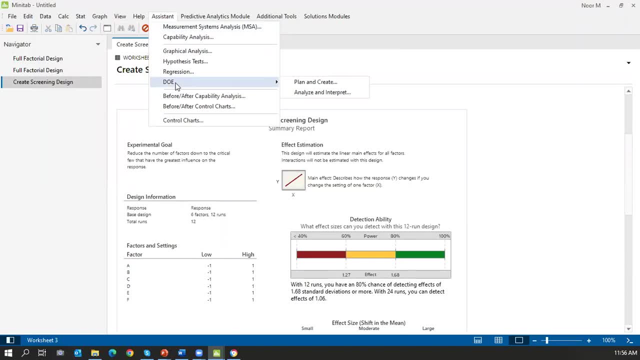 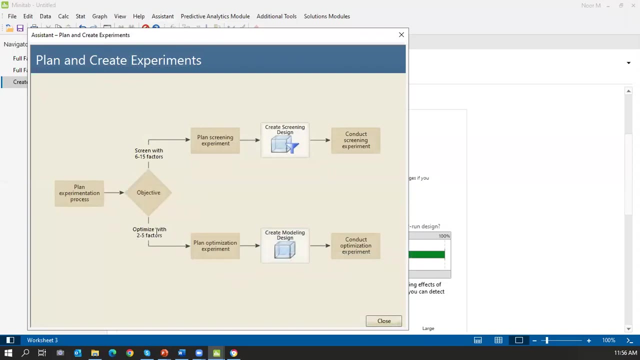 Okay, but For the assistant, have a limitation on that: Only five. factor for the four: factorial: Okay, if let's say you go for this case, plan and direct here Here is a plan Okay, create design itself, So they will. assistant already put here. optimize only two, two, five factorial. 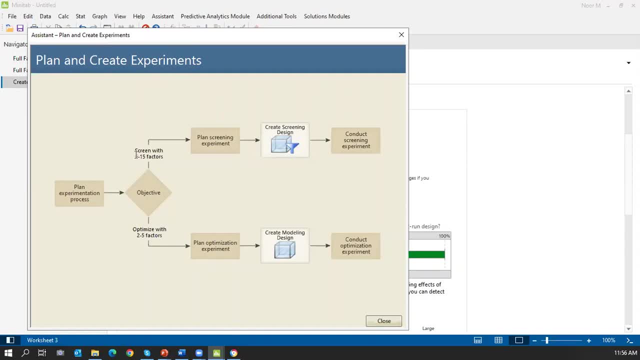 Okay. so if let's say for the screening part they only goes up to six, Okay, we start six. up to One five factor. So this one is a limitation. If let's say you have more than that, you can go for the stat DOE. 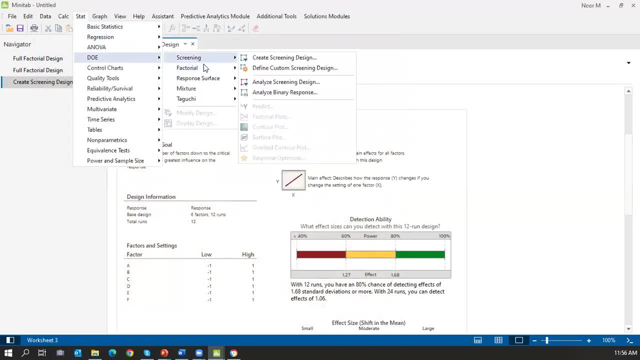 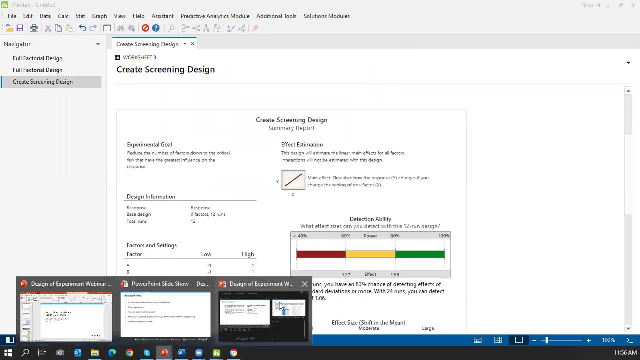 So go further, maybe factorial, maybe screening factorial, maybe the response, factorial and mixture design, and then the gucci design. Okay, so I will back to this one till you finish all this. Okay, so do you have any question? 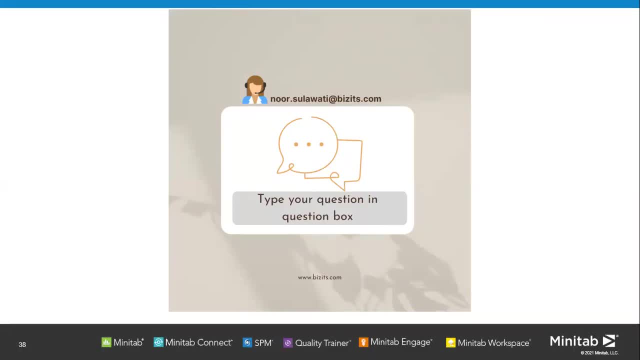 So if let's say have a question, let me know, Okay, I will share this material. So you put your email in the chatbot or Q&A bot. I think it's a chat in chatbot. So I will email after this. 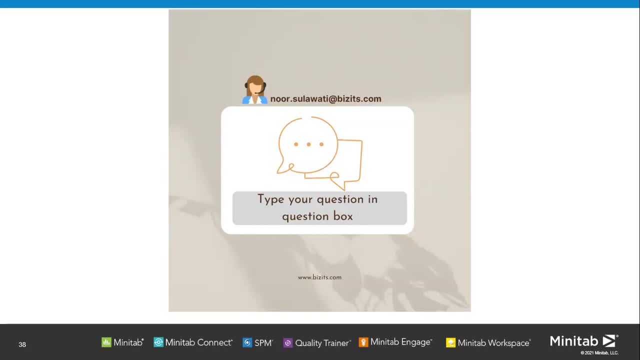 Okay. so this one is a good question. It's a. which, which is a DOE, is better to use for parameter optimizer: full factorial or response surface? factorial, Okay, response surface. So this one is a. depends on your situation, Okay, depends on your factor, depends on your response itself. 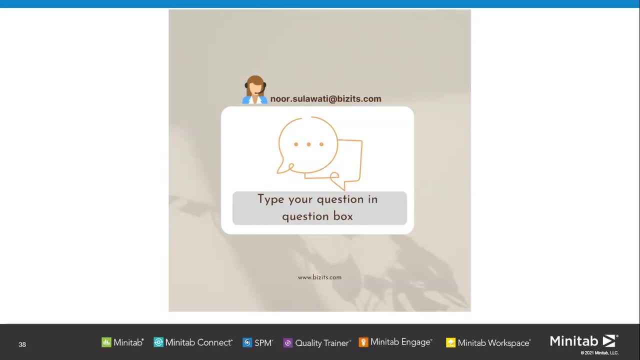 Okay, it's not. this case is not, will be the good one, is something that one, that one know. it will depends on your situation, It will depends on your factor, it will depend on your level and then, of course, it will depends on your costing. 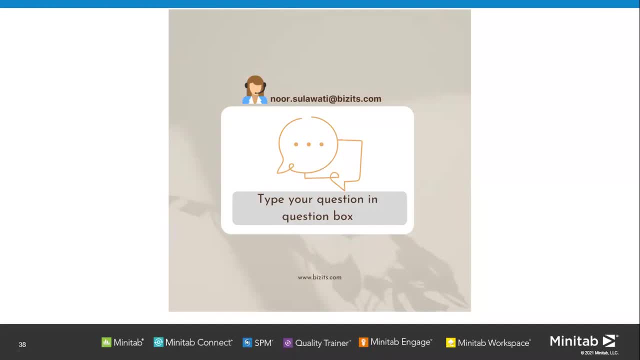 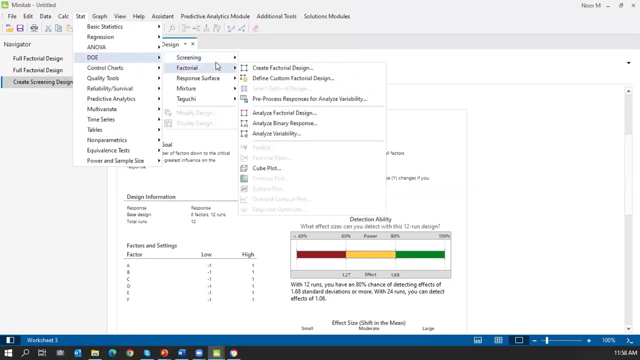 So that's why we have a lot tie of the design itself. Okay, today I will just show on the design, full factorial design. So you come back to the start. DOE, maybe you can go for the screening part first and then, after the screen part five, you go for the factorial. 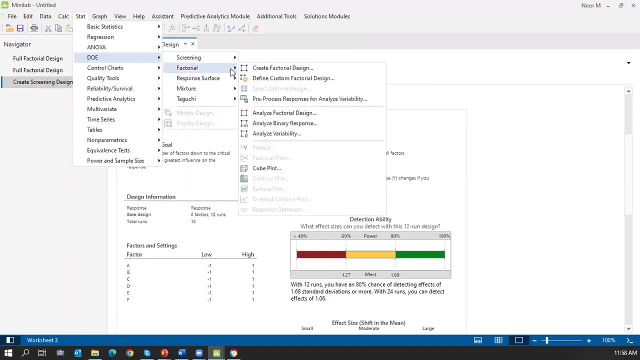 Okay, but Your your about the limitation. maybe you can go for the response, you can go for the fractional only and then maybe if let's say your, your, your Y is not the straight line, maybe the response surface, it will be the best way. 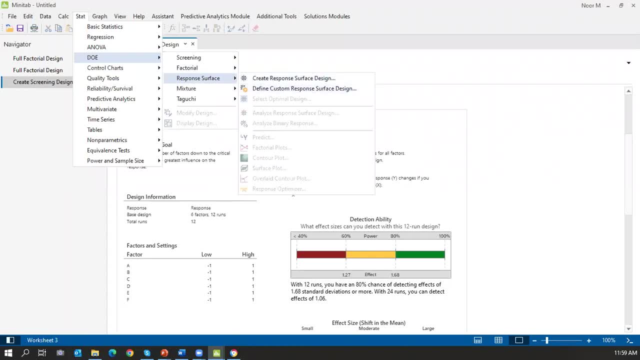 Okay, for sure, I think, the real life one. I think most of you will use the response: surface design. Okay, which is the best is depend. Okay, hopefully I'm clear. Answer your question. Okay, so we have this question. 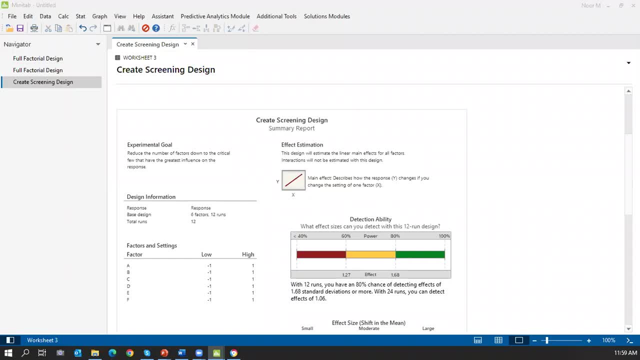 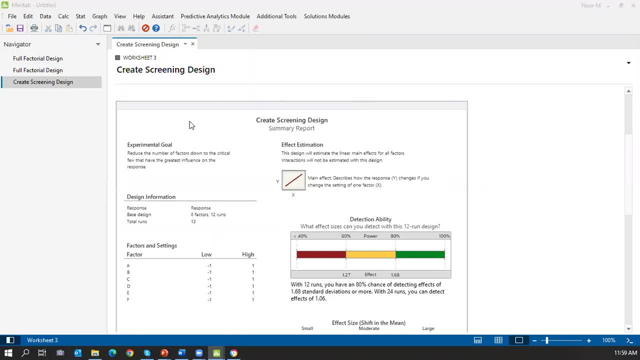 Yes, can. they will have that one in by the Traffic. if, let's say you have the, the, why it is are not measurement is as something like tax. you can go back to just add: Yes, can, can, can, can. steps for you can go for the factor design and then you just binary. 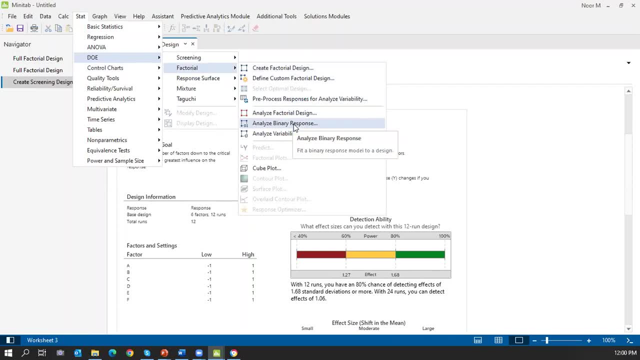 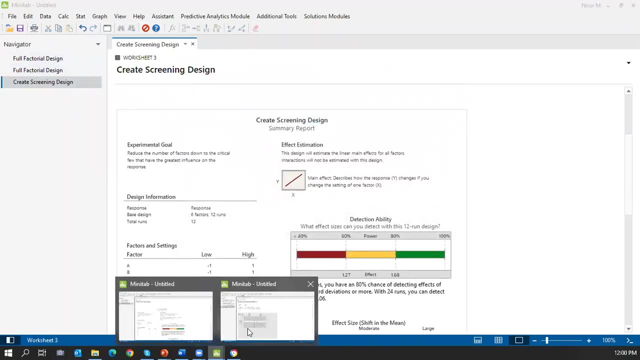 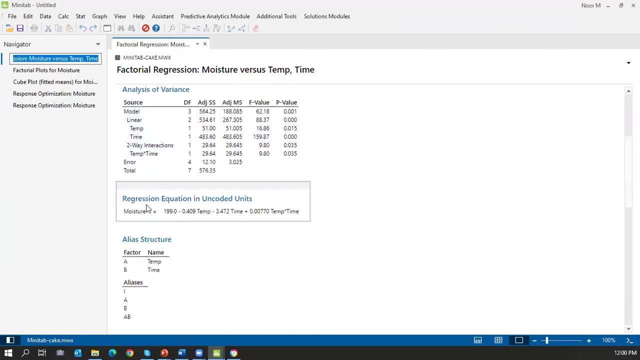 Yes, In municipalities, say, you have a two option only. this is on, not delicious, So maybe it will be different in term. Yeah, It was a friend in thumb anova here. okay. and then the the regression line here. okay, we not use the regression, maybe we'll. 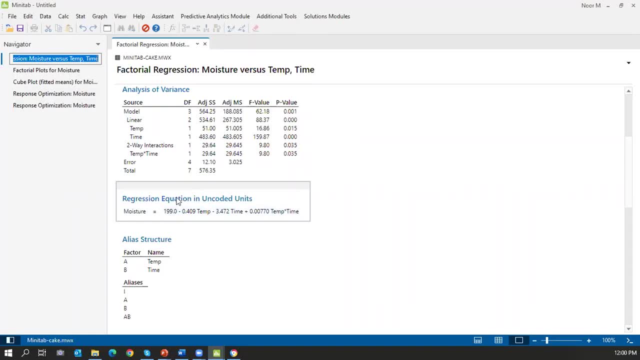 use the logistic regression, something that one just different method. method only, the objectives is the same. okay, hopefully answer your question. if the response is defective percentage, how to perform? defective percentage means meaning that it's a measurement, is it okay? so if let's say measurement, it still will. still will the same.